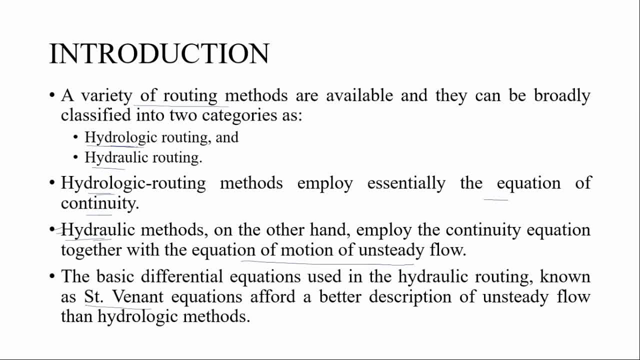 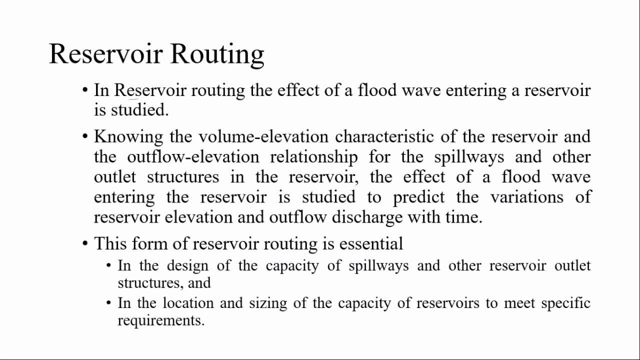 Centrivalent equation and the contrived momentum equation. Of course, these are used for the unsteady flow In reservoir routing. when you talk about the reservoir routing, what we do is the effect of flood wave entering reservoir is steady, So it is steady. If flood wave is entering reservoir, you want to predict what's going to be the discharge or the elevation. 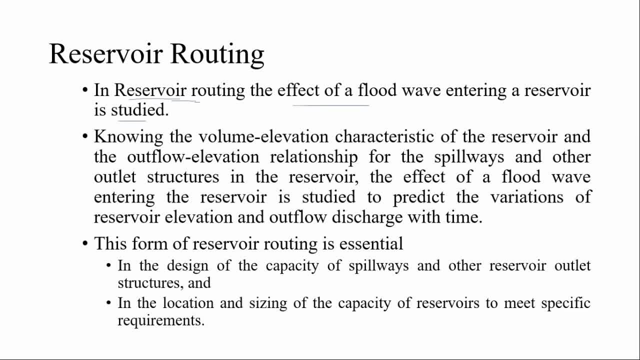 of the reservoir. Some things are known to us that if the volume elevation characteristic is known to us for the reservoir, How the volume shift, So this can be known by the area, base area of the reservoir, Outflow elevation. so so outflow discharge is occurring based on the elevation. you can establish a relationship to the spill way or anyきた. 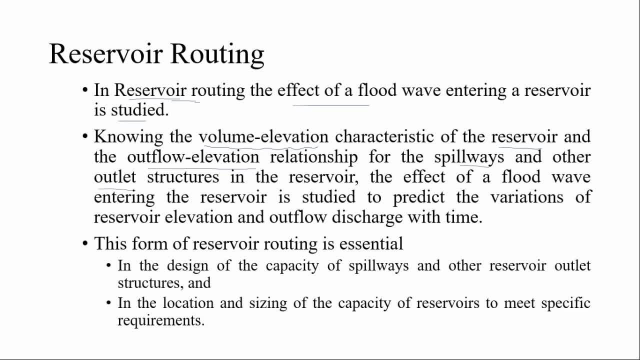 other outlet structure, then the effect of flood wave entering the reservoir is studied. so we want to study the effect. so let's say this: in front is coming and in the reservoir, if a flood is occurring, you want to know, study its effect, you want to predict the variation of. 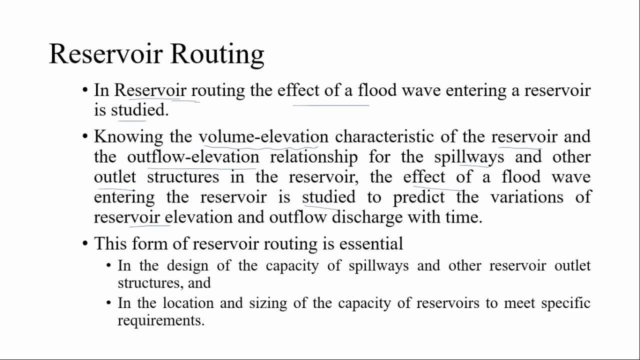 reservoir how the elevation of the outlet discharge will change if some kind of flood occurs in the reservoir that enters the reservoir. so this is basically. we use it for the designing of the capacity of the spillways or the, or the location and sizing of the capacity of reservoirs. 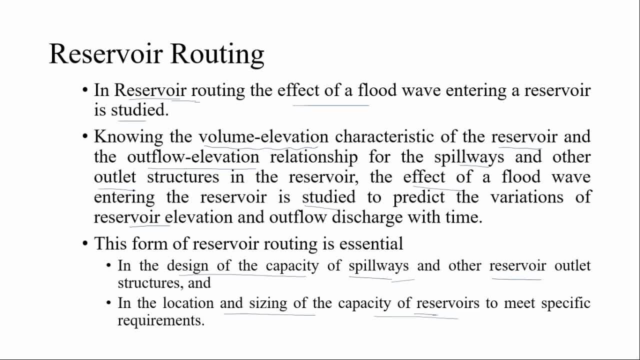 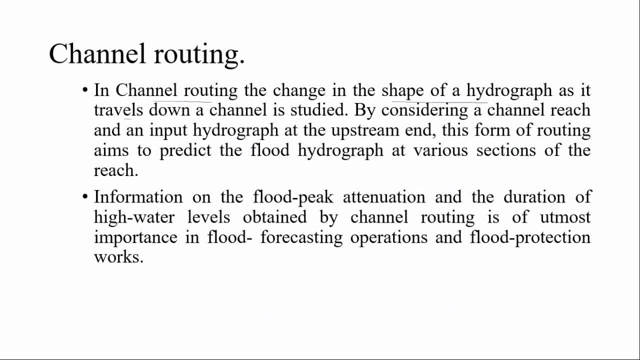 and mostly spillways and reservoirs. there is a channel routing when we use we use it to find the shape of the hydrograph as it travels down the channel. so different, different sections consider that there is a various section and for each section we have had the channel routing and find. 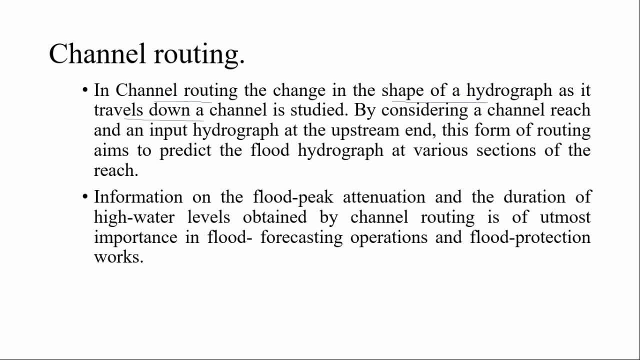 the shape of the hydrograph. so this form of routing aims to predict the flood hydrograph at various sections of the reach. information of the flood, peak, attenuation and the duration of high water levels obtained by channel routing is of most importance, so we are trying to predict the flood. 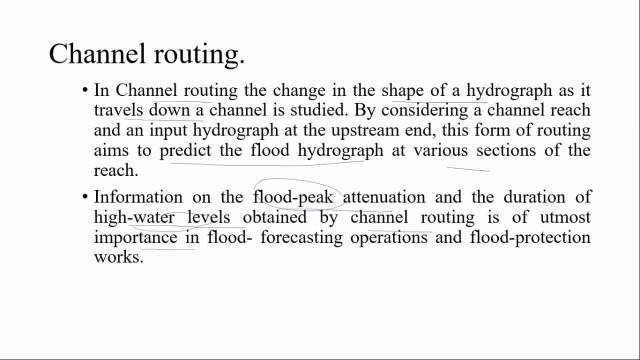 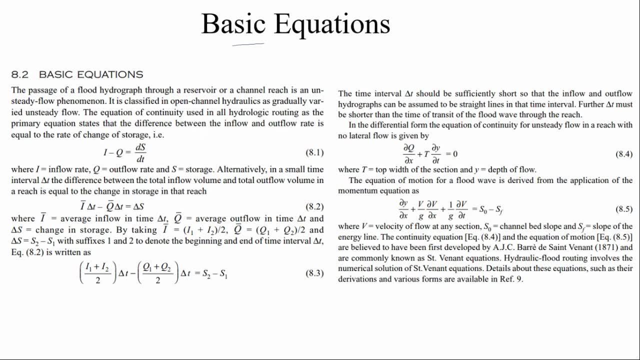 peak and attenuation or the high water levels in the channel. so this will enable us to do the forecasting, for forecasting or flood protection works now from some basic equation that we using. so the passage of flood hydrograph to reservoir or channel is an unsteady phenomena. yes, we know that. 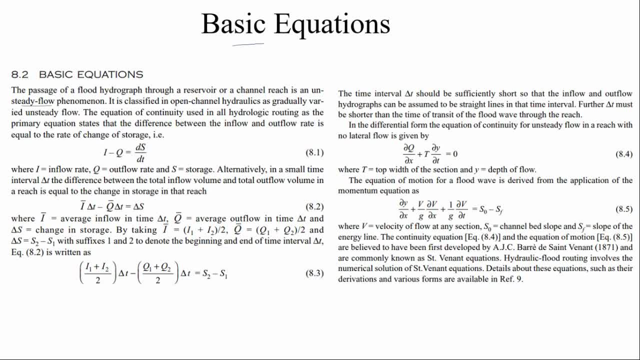 it is classified in open channel hydrics as gradually varied unsteady flow, so it rapidly vary unsteady flow gradually. so rapidly means usually we consider low hydric jump. so it gradually means slowly, it is changing gradually. the basic continuity equation that we use in hydric routing is simple. 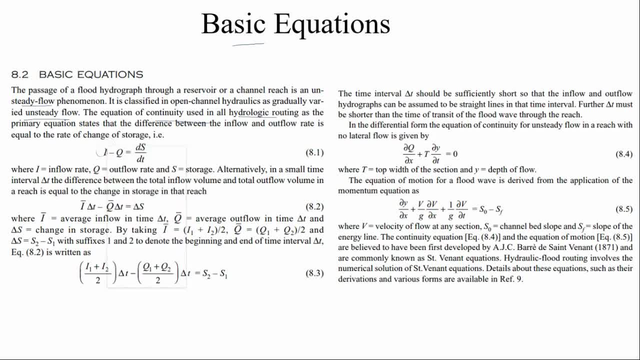 here. so rate of inflow, inflow minus outflow, is equal to change in the discharge for given time. so i is the inflow rate, u is the outflow rate, s is the storage and dt or the delta, t is your time. okay, so if we consider all this, if i cross, multiply it, what will i get? average inflow into delta time? 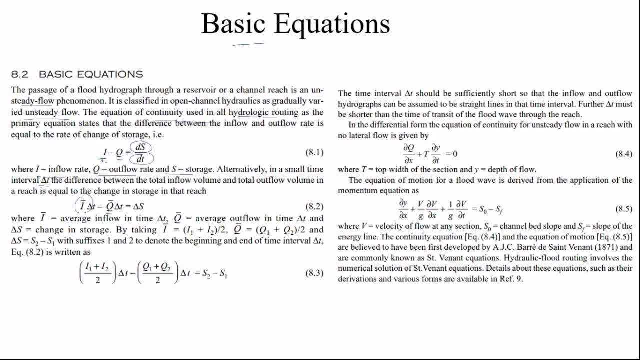 minus average outflow into delta t, dt. i have written approximately delta t, so what will this be? i delta t minus q delta t equals to ds, where i is nothing but average inflow. that is the i1 plus i2. i1- previous step back. i2- next step back. this time i am calculating. 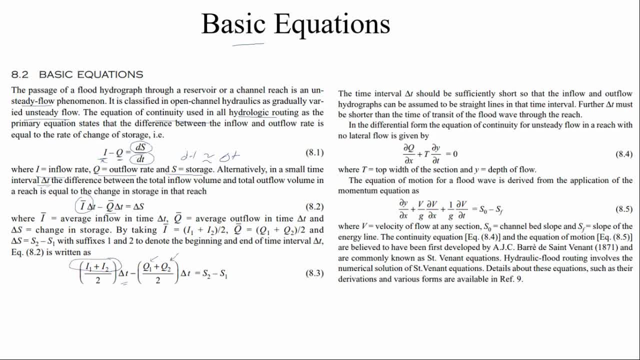 similarly it goes for the q1 and q2. delta t is the time factor, delta s but the difference of s2 minus s1, that is a change in the storage, if we talk about some other equations, which is a little complicated in differential form. so this continuity equation, this continuity equation, you can write in the form of: 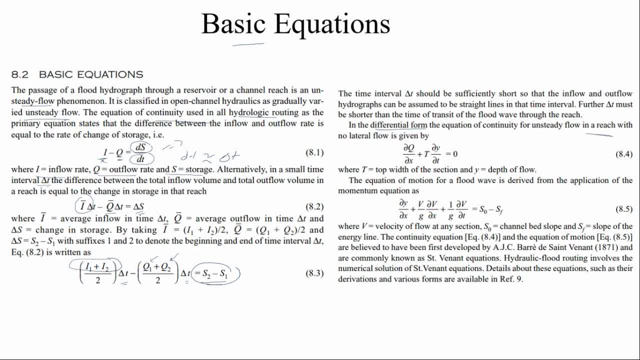 in the reach, basically in the reach for a reach, when there is no lateral flow. if we consider this, then it happens. this is 1d. of course, this is basically 1d. equation x is what we have to consider, so we will. 尴q, x, x. t is the쳐ft width of. 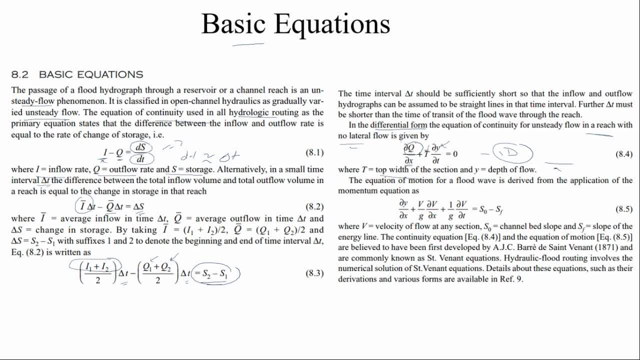 vol, Hyp momentum equation. this is y, x, v is the velocity of this flow. V, x, g, V, T, x turns ing. this is not the storage. so s0 is a bad slope and sf is the momentum energy line slope or the sf energy slope. now again, i said this is the sand planet equations, so these equations are mostly 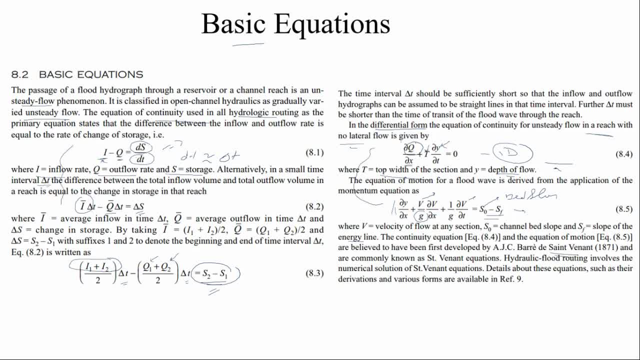 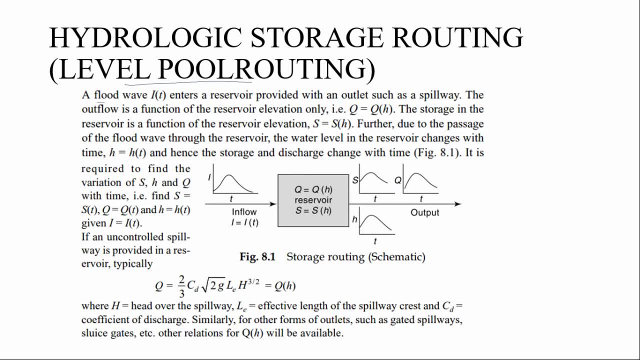 used in hydraulic routing and these equations are mostly used in hydrologic routing. now, first method is level pool routing. now let's see again. we have a flood wave like this. it enters the reservoir, that's, it is a reservoir with an outlet. the outflow is a function of the reservoir elevation. only, of course, q is a function of. 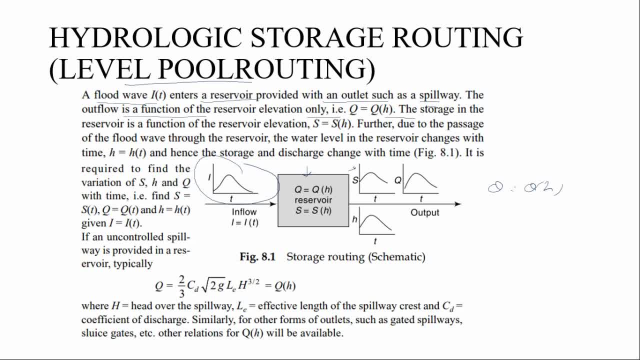 height right. the storage in the reservoir is a function of elevation, so storage b, h function. so sb function, h or qb function. the water level in the reservoir changes with time because this is changing with time in flow hydrograph. so the water level h will be a function of time. it depends on the time. so what does this mean? this means that 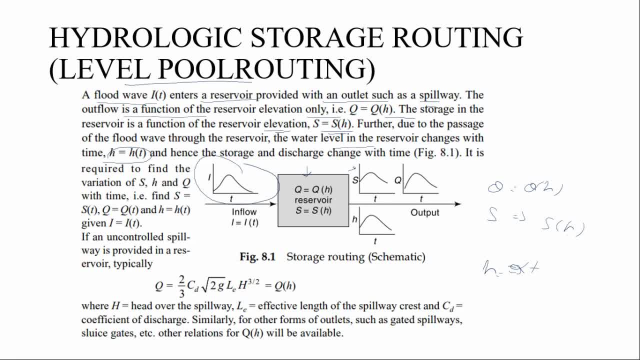 q is h function, sb is h function and h is basically t function. so q and s both are time function. so q and h will change with time. they will change with time because the inflow is changing with time. now let's say, i is a function of time, h is a function of time, so q will also become function of time. 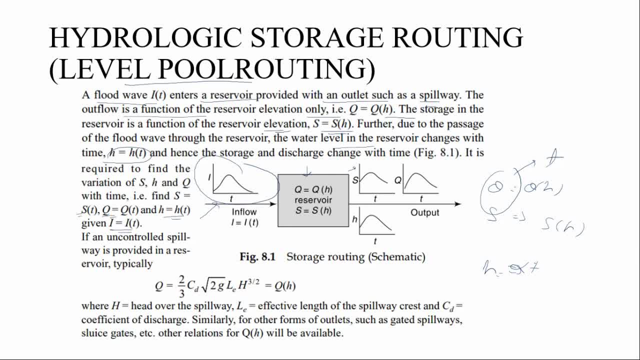 is also a function of time. so everything is a function of time. okay, simple. now, uh q is a function of time. now, uh q is a function of time. we know that if we talk about the spillway, we know that, if we talk about the spillway, so we know that q equals to 2 by 3 times. cd is the. 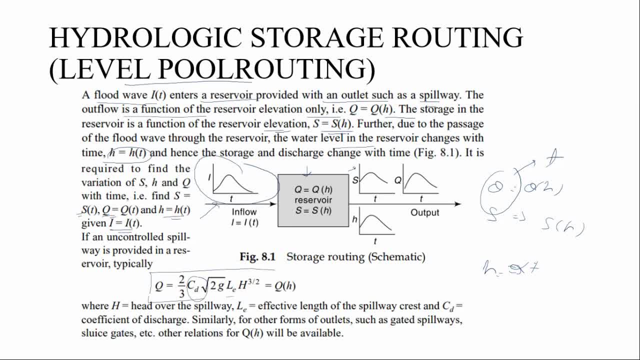 coefficient of discharge root: 2 g. l is the effective length of the spillway, h is the head over the spillway. this is mostly used in various spillways like v-notch, rectangular, notch rectangular, v-notch, rectangular v-notch, etc. we have a clear elevation, so this is how it works. what do we need if we are doing reservoir routing? 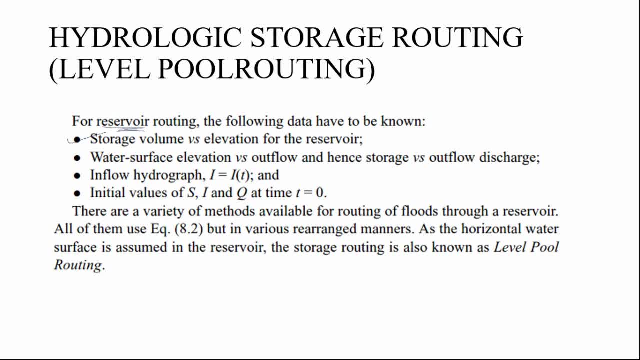 so we need storage volume versus elevation. we need this relationship. we need water surface elevation versus outflow. we need inflow hydrograph. okay, this is all we need. and initial value- very important. we need initial value at the initial stage. how much is s, how much is i, how much is q? 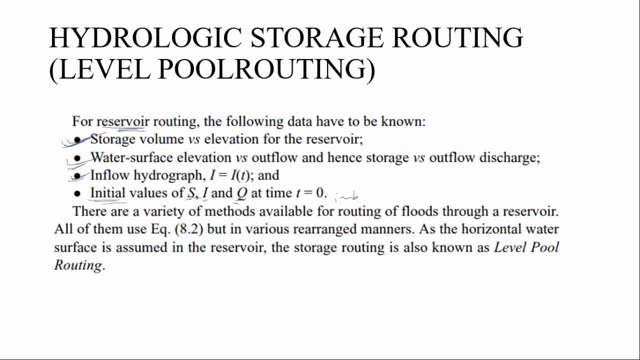 only then we will be able to move it forward. so this method is called level pool routing. okay, uh, as the horizontal water surface is assumed in the reservoir, the storage routing is known as level pool routing. so we have to consider the horizontal water surface as the reservoir. 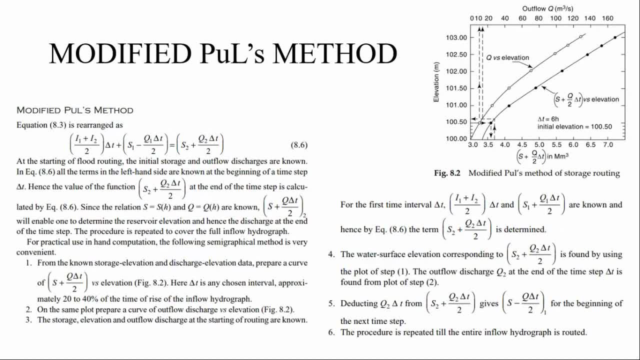 we don't have to consider any other shape. it is spelled out with the. then there is a method called modified pulse method. so what do we do in this? we had the same equation. so what was the equation? we had i1 plus i2 by 2. 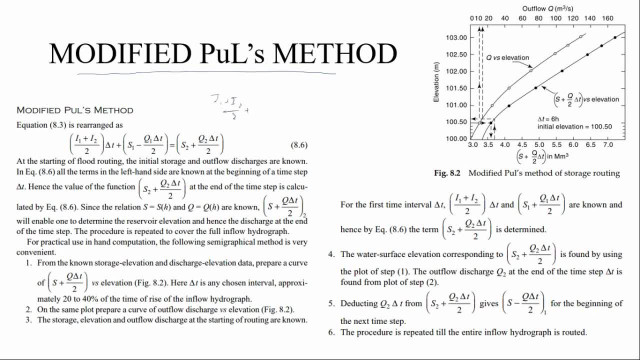 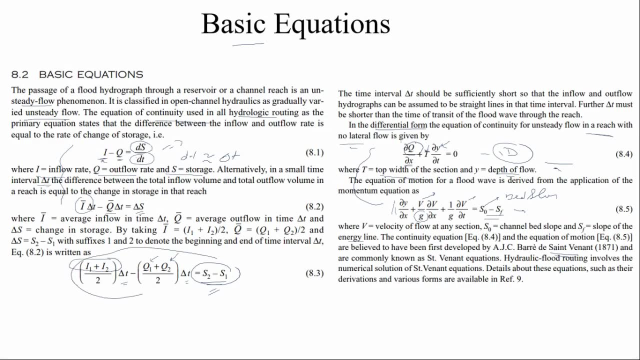 plus uh. we had uh. q1 plus q2 by 2 is 2 minus s1 multiplied by delta t, of course. so this was the equation: we had: i1 plus i2 by 2 delta t minus q1 plus q2 by 2 delta t equals. 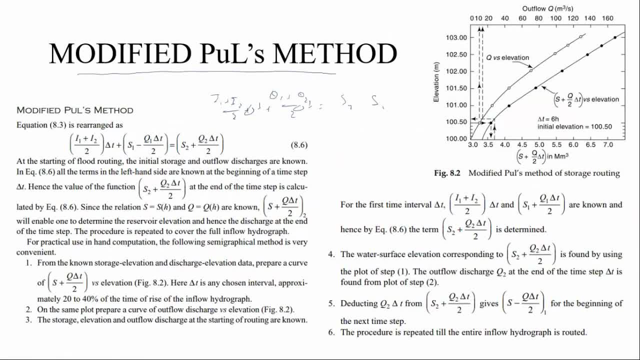 s2 minus s1. you change it in this form and do this with this equation. same what we did here. we kept q1 and s1 together. so if s1 minus q,1 plus q2 plus s2, equal to s1 in this form: 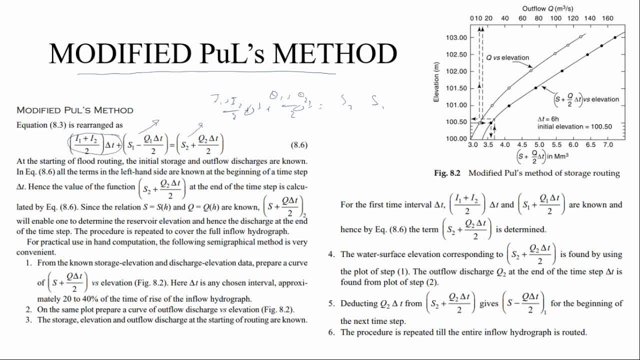 Q1 delta T by 2 is one term and S2 is equal to Q2. Now see, we know I1 plus I2 by 2. We know S1 in the initial stage and Q1 in the initial stage. This is unknown thing, So let's see how it works. 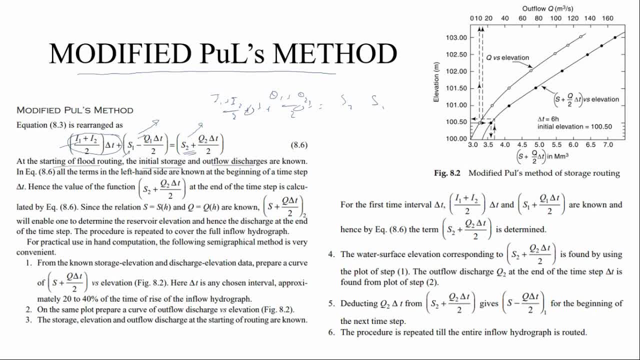 Starting of a fuller routing. the initial storage and output discharge is known, So we always know I1 and I2. We know Q1 and S1. All the terms of the left side are known. So basically, we know all these. What is unknown? Only this. 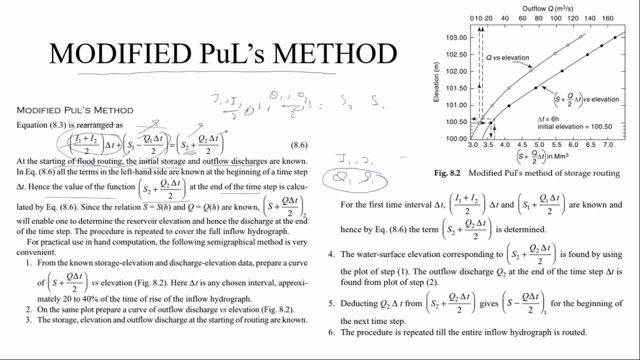 The value of the function. this, at the end of the time step, can be calculated, Since the relation of this and this are known. So we know S is a function of height and Q is also a function of elevation. What can we get out of this? S is also a function of height, Q is also a function of height. delta T is a constant. 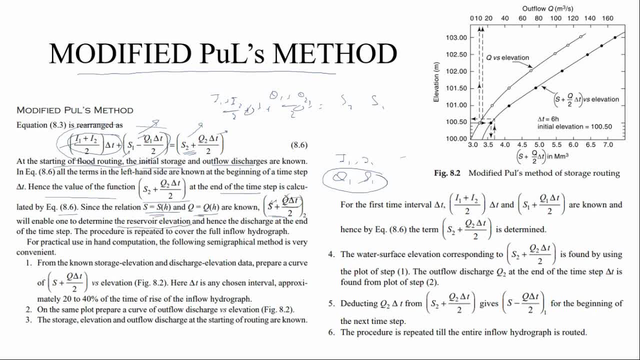 What can we get out of this Reservoir elevation or the discharge? We can get out the reserve elevation and discharge from this full term. Now we have given a step by step procedure From the known storage elevation and discharge, prepare a curve, So this curve is made. 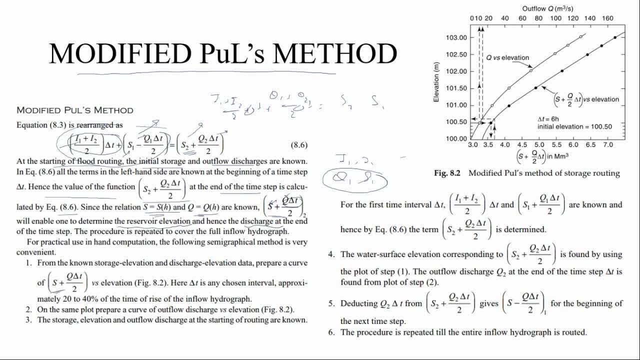 Which curve is this? This is elevation on Y axis and they have put the S plus delta T into Q by 2 on the X axis. So this curve is made S plus Q by 2 into delta T. Along with this they have given the curve of Q versus elevation. 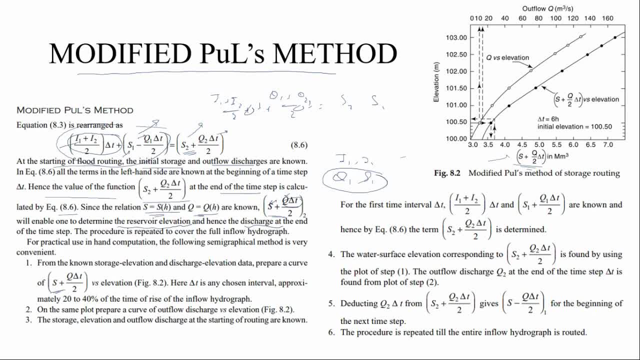 So we can make a curve or we can keep a table of form of this data In which elevation will be there, Elevation will be there and Q will be there, Or Q plus S by S plus Q by 2, delta T will be there. So, anyways, we just want a relationship between elevation and all these terms. 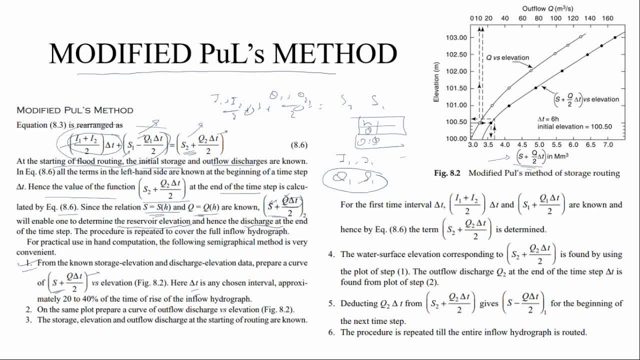 We assume delta T is a little small, Usually 20 to 40% of the time of rise of the inflow hydrograph. On the same plot we have shown the discharge and elevation. The storage elevation and outflow discharge at starting of routing are known Just like that. 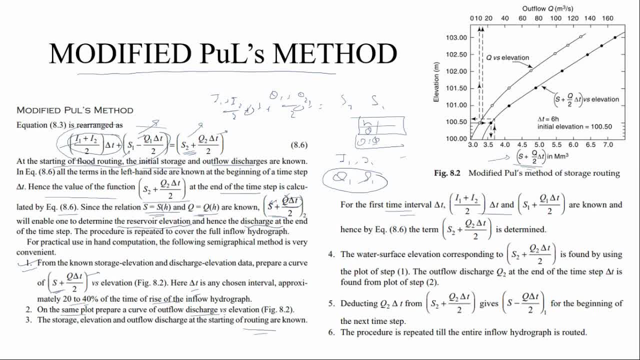 First time interval: delta T. we know this, So we will remove this. We have removed this at the first time step. As soon as we get this, What can we do? We can remove the outflow discharge from this Because from this quantity S plus Q, delta T by 2. 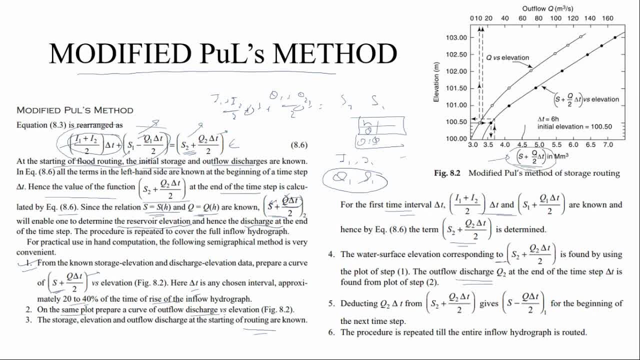 What will we remove? We will remove elevation. Suppose this is our 4.55. I have removed elevation from this curve. I got elevation 101 point. Now I also got the corresponding rate of this 101 point, Which is elevation. So I will also get the discharge from this curve. 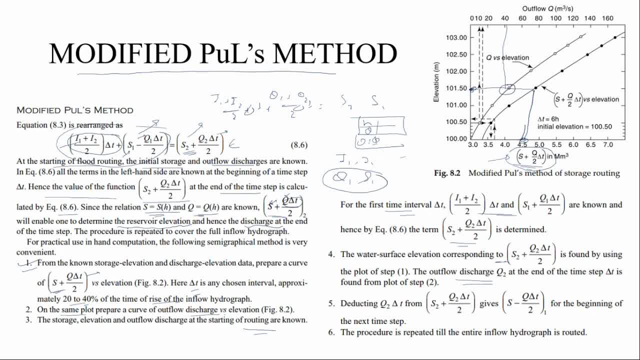 Which is 0.40 Once again. So I assume 5.5 is my S plus Q delta T by 2 delta T. I go from here and put my hand on this curve, Then I get elevation from here. As soon as I get elevation, I know I cut this graph here. 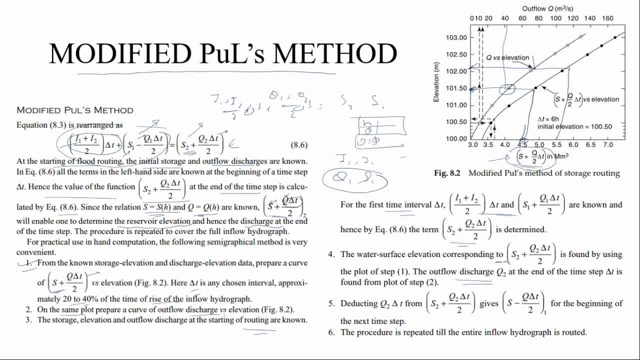 I will get the corresponding discharge from this elevation, from this curve, And I will also get the discharge from here. So this process you can follow, Or you can also do interpolation, If you have data, So you have the value of this in the table form. So between these two values, 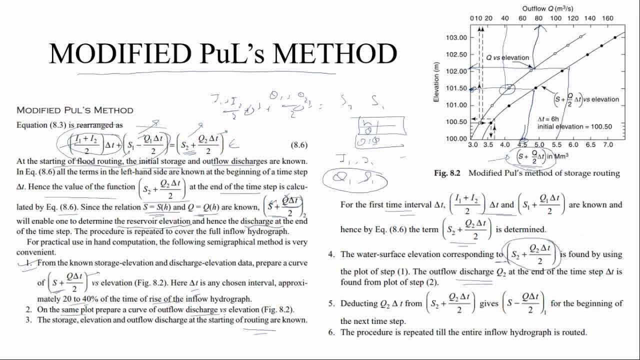 You can take these two values And accurately predict the elevation And with that accurately predicted value, You can interpolate and accurately predict the Q, So directing. Now, once you have this value, What do we need for the next step? We need this: S minus Q, delta T by 2: 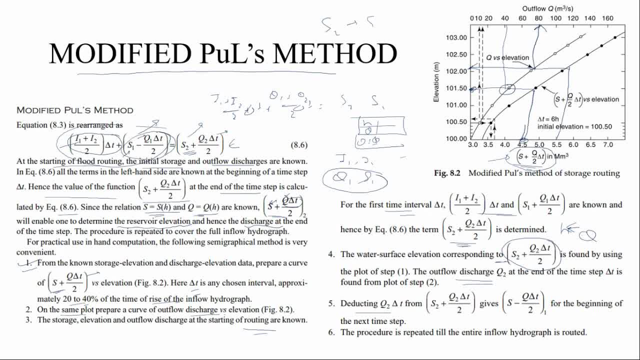 So your S2 will be the ultimate S2 And Q2 will become your Q1. But you have to change it to this form. So if I subtract this quantity Q2 delta T, Then this quantity will become this. It is arithmetic And we will repeat this process. 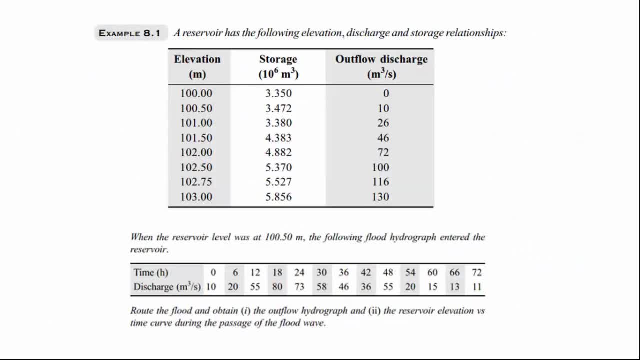 Until we get the final result. I have given an example in this book On different, different elevation, Different storage S and Outward discharge Q is given. One more thing is given here. I have given the initial level of the reservoir, That is, I have given H1. What is it initially? 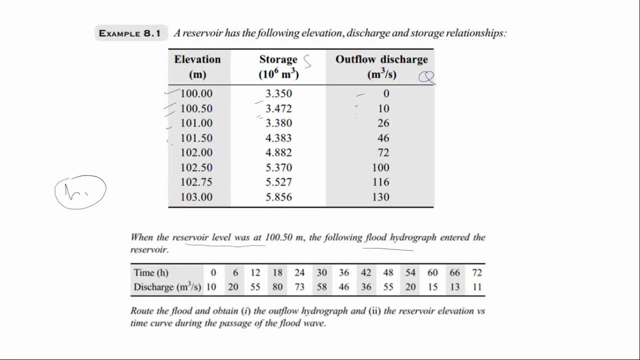 I have given the entry of the flood hydrograph. That is. This is our I. This is the discharge I. This is our Q on the outflow. So I have given discharge on different time steps. I have given I. I have to get outflow hydrograph And reservoir elevation versus time curve. 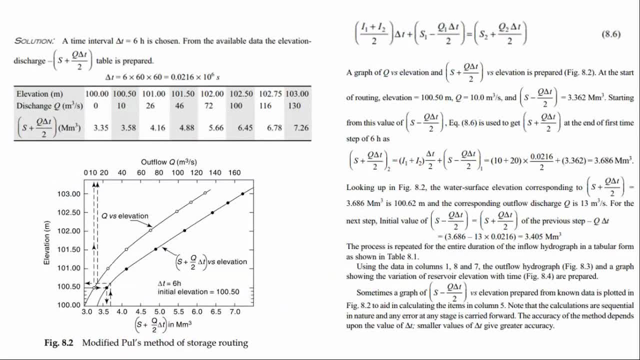 I have to get these two things, Ok. So what will we do? first, As I said, We have chosen delta T for 6 hours. Now, from this delta T, We have to establish a relationship. What is that relationship? That is S plus Q, delta T by 2. 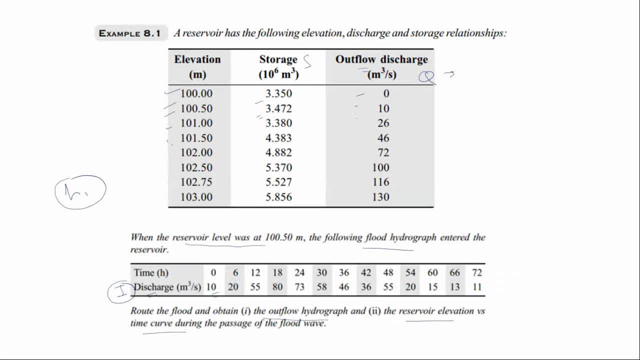 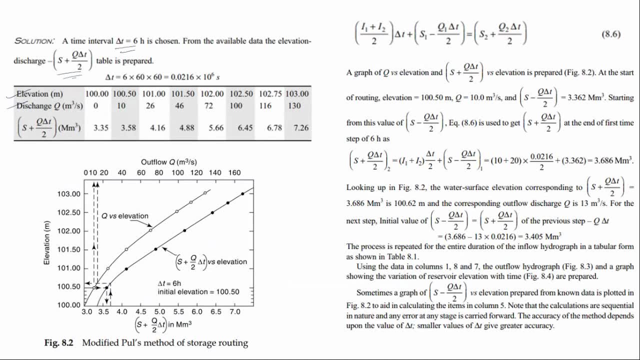 Elevation discharge is given to us. Elevation discharge is given to us. What we are doing is S plus Q. delta T by 2 is taken out, So let's say 3.35. How will it be? You can check that. So for the first step, 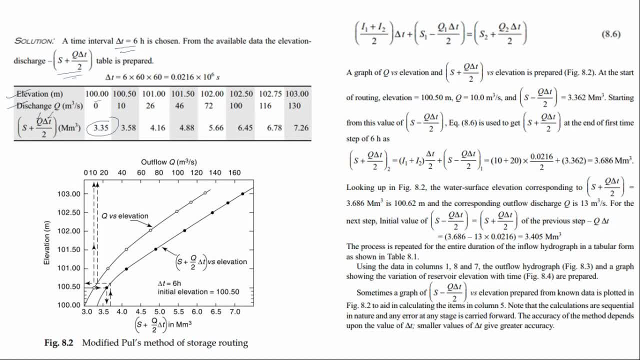 For this elevation, Q is 0. Delta T has no use. S? What is S? 3.35? It simply comes as 3.35. This is 10. So S? How much is S? S is 3.472. So what you are going to do is: 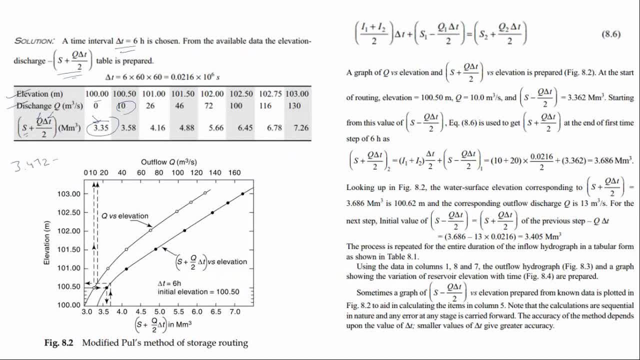 3.472 Plus your Q, And that point is 10 Into delta T. You can convert this into second. Now this is of course in million Metre cube, So into times power 6 Plus 10 Into 0.0216 Into times power 6. 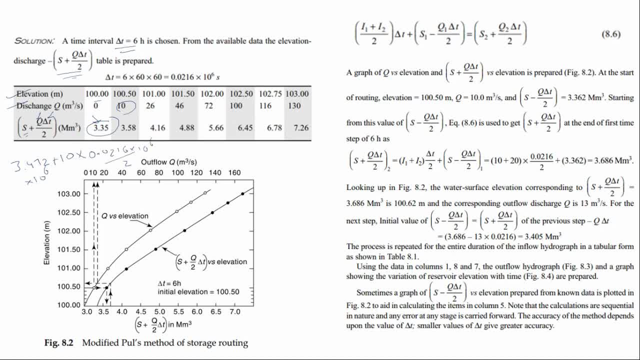 Upon 2. So when you add this thing here, You will definitely see that It is going to become 10 here. So this is going to be 0.2 And this is going to be 2 from 0.2. So this is going to be 0.1. 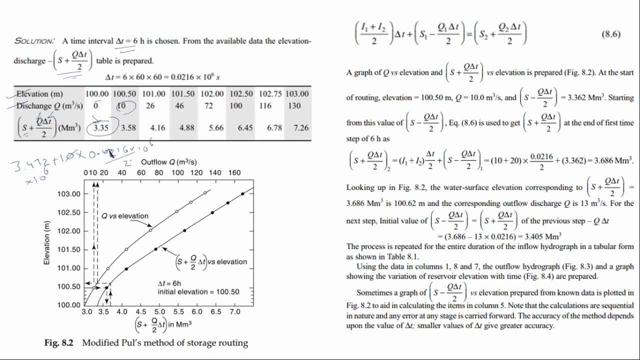 So 3.472 Plus 0.1. If we do, Then here about 3.57 Is coming 3.58, So You can do this table. Ok, So Let me Erase all this So this can be Done easily. And now what? Now you can see. 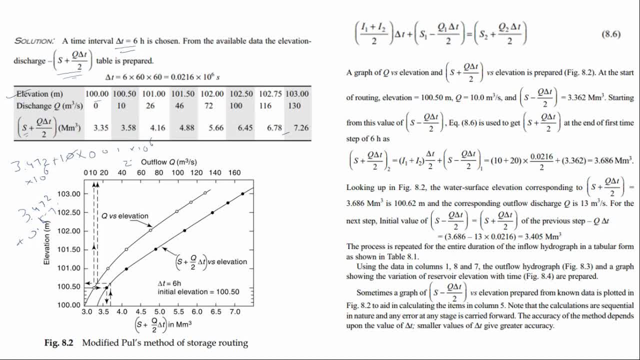 That You can see That. You can see That This, This Curve, Is made To show. So without The curve also, You can solve this question, And this is the equation That we are going to use Now. So We are done Now. one thing important is That: 100.50. 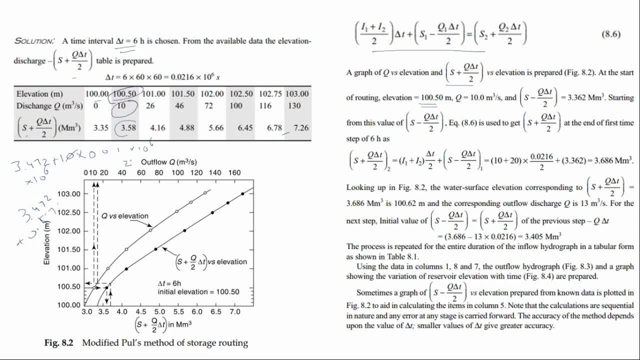 We have given initial, So initial Is given For that. Initial Q1 is 10 And It will be This much. So we have given Initial Q. We need quantity 1, I1 Plus I2, 1, 6- see, all the units are in million meter cube, so no need to worry then we 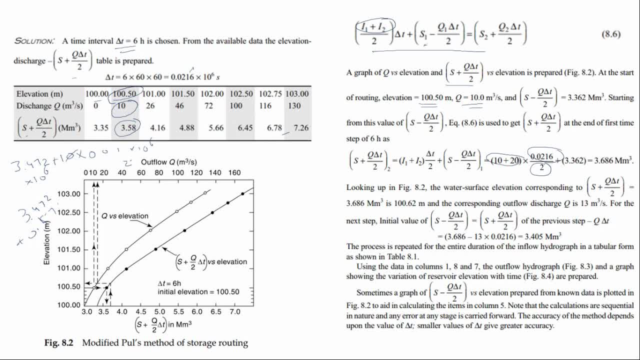 need s1. s1 is 3.47 now, okay, so they have an article. this s1 minus q delta t by 2. yeah, so what they have done. so if you do it in the in this manner, you have s1 is 3.47 to 3.47 to minus q delta t by 2, minus point to q 10 into. 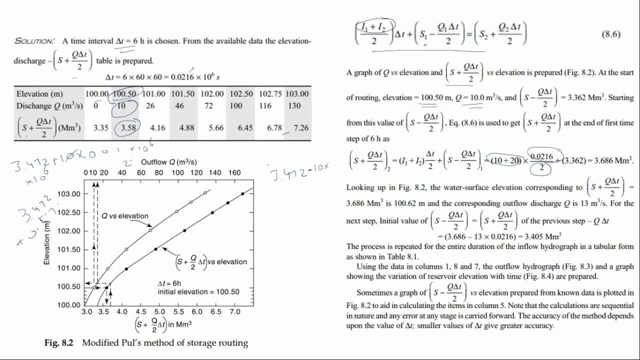 whatever conclusion we have done here, it will become the same. so 3.47 to minus 0.1. 1 to something. 1 to something, so 3.36. this is what they are getting here. are you getting my point? so discharge this time is my discharge for a minus one equation with delta t pixel as given. 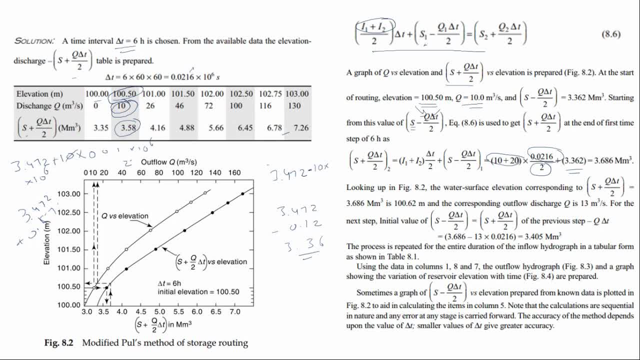 score a chemical 3.36 to real gap. so this becomes my s plus q delta t by 2, now 3.686. now what you can do is, with this 3.686, you go up the graph, find the elevation. so what evaluation you get? elevation will uncle hundred point six. 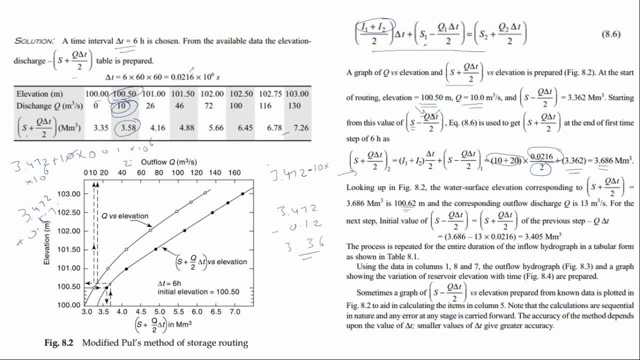 two, so you can see this value. you can also calculate from these two values. so hundred point five, pay up a hat. three point five, eight, two point here, or hundred, one pair of four point one, six, three point six, eight, six, two half, and each one here: three point five, eight, six, three point six, eight, six. and we do 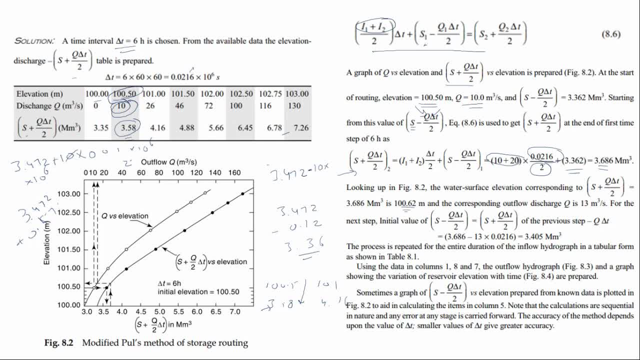 totally dang it. two hundred point five, so total design at one point six two go, so you reaching up to hundred point six two, and similarly four hundred point six two is charged up. interpolation curse at the home. excuse me, that is also coming up to be thirteen between these two, sorry ten and twenty-six, is it going to be 30 meter? 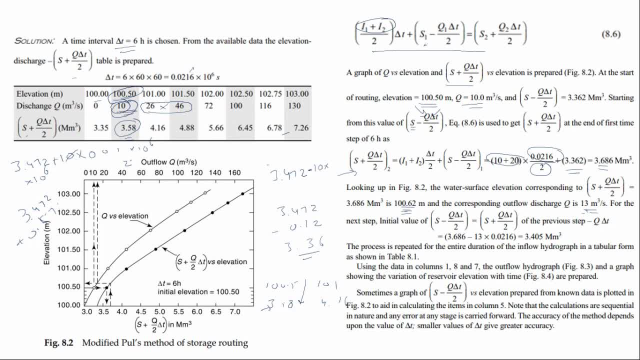 cube per second. so the same thing can be term, using it, table of force. so for the next step now, other up was value, as you subtract minus Q duty from this value, so you get three point six, eight, six minus thirteen times point zero two. it's over six thirteen q. that is the cue. they will just power. 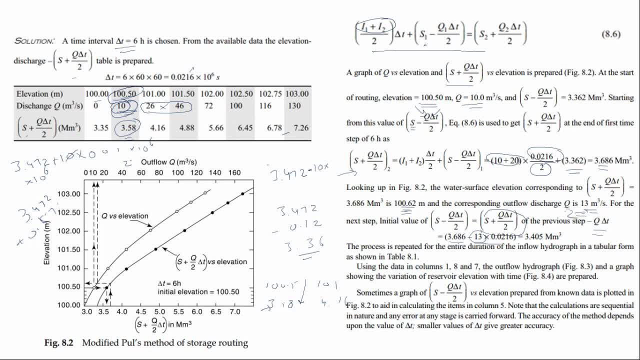 this is it. Q 2. so subtract E, I multiply it by your delta t, by 2.. So delta t, not delta t, just delta t, you get 3.405.. So you repeat this process, you get this kind of table. So all these times you know one: these inflows are: 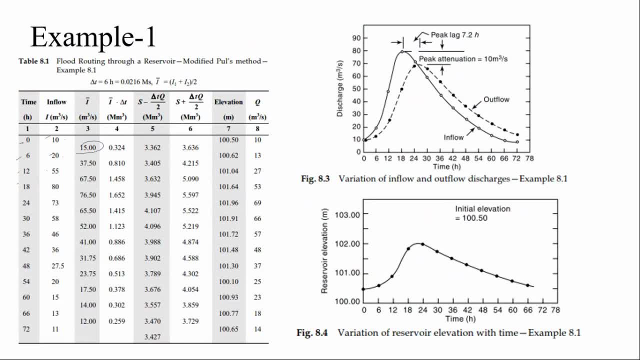 no one: i1 plus i2 by 2, 15,, 20 plus 55 by 2, 37.5,. multiply it by delta t 0.0216,. you get this value Now s minus delta t cube by 2, so this also you can calculate and s. 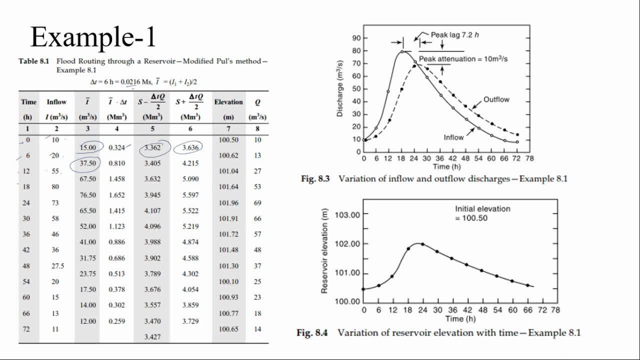 plus delta t cube by 2, using the equation you can calculate, And again using the relationship or the curve, you can get this value 100.62.. Now this becomes from this s plus delta t cube by 2, you again get the 3.405 and you get, ultimately you get the 4.215 using this. 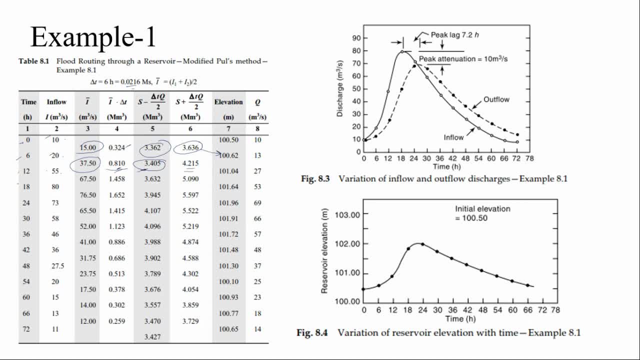 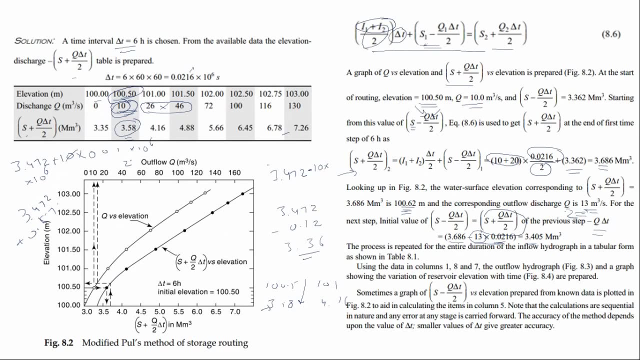 value 0.816,. using the new value of this s minus a, this one, You get pretty straightforward. So is there any doubt? See here, this value is nothing but average value into delta t plus this negative value. you add, you get this value: Average value into delta t plus this. 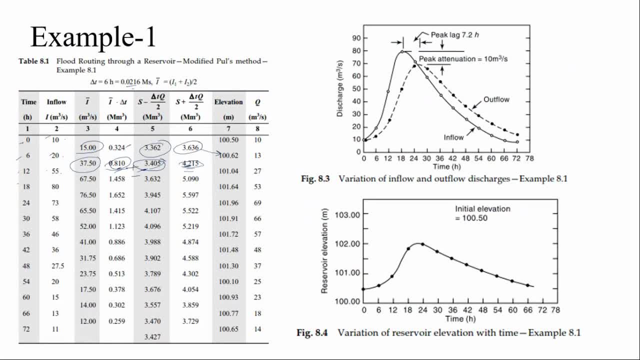 value. So, basically, this column is nothing but sum of these two values. So you get these two values and, finding this value from this s plus something, you get it by the elevation. from the elevation, you get the 3.405.. 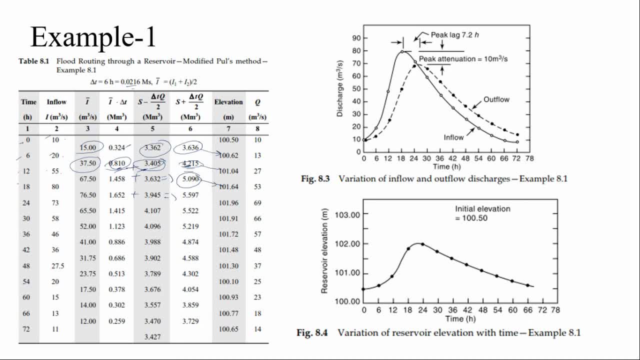 So this is the discharge. this also you can get from the elevation curve, and subtracting the discharge plus discharge into delta t, you get again this new value. So this goes like this: So you get this value, you get this value. So this goes on. So this was. 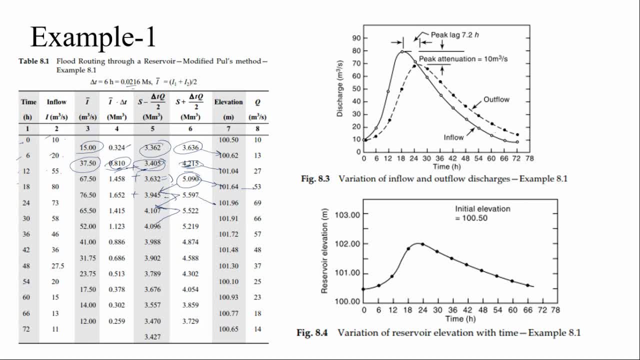 the inflow hydrograph and with that we also have the outflow hydrograph, So peaking somewhere near this 24.. So there is of course a time lag: 73 or 69.. So there is also time lag and it is 80, of course for this case. And this is the variation. 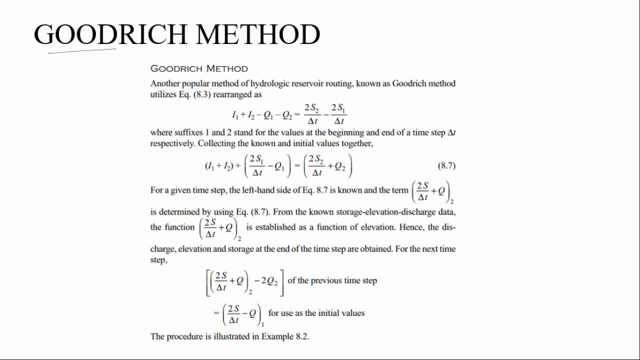 of the time and elevation. Now there is another method, Goodyear method. there is not much difference between those two methods. Little difference is of that. it has difference to write, In that case, what was said- psi was one term and also omit that two and multiply. 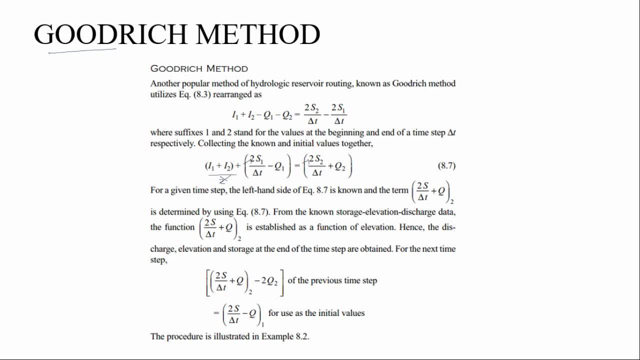 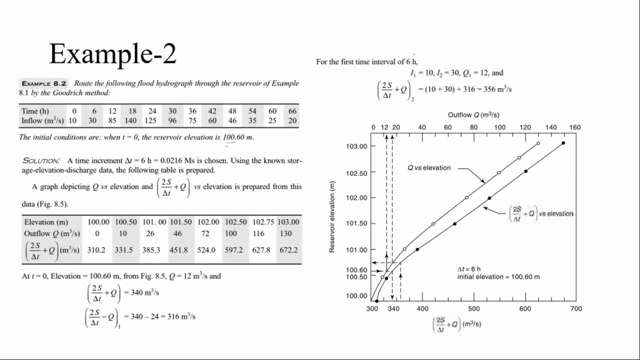 over here. So this is Goodyear method and took no difference. The same thing you are doing … … … … … … … … …. So all other things are same. instead of every value, you are just adding these two values. Same example given here, except this time elevation difference is given. 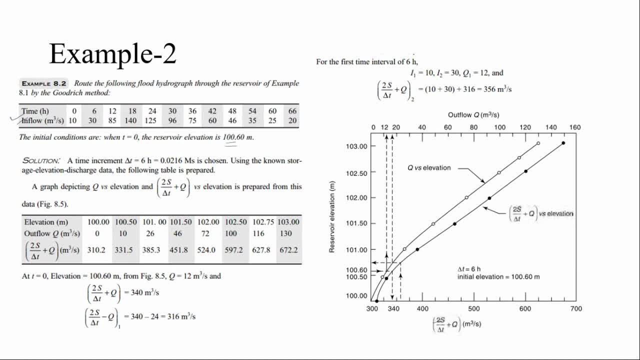 In this 2s is given and s plus q. delta t divided by 2 is just a little difference. Delta t term was here and delta t term was here, So I think well understood. So you see, here You have plotted a graph of q versus elevation and it is 2s by delta t plus q. 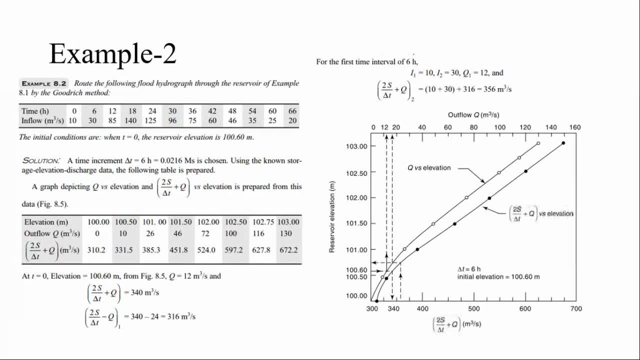 Yeah, so let's, let's look at the example also. So this table: you can prepare 2s by delta t plus q, given the q and s s is the same. So this table I think should be a problem because delta t is same: 0.0216 million seconds. 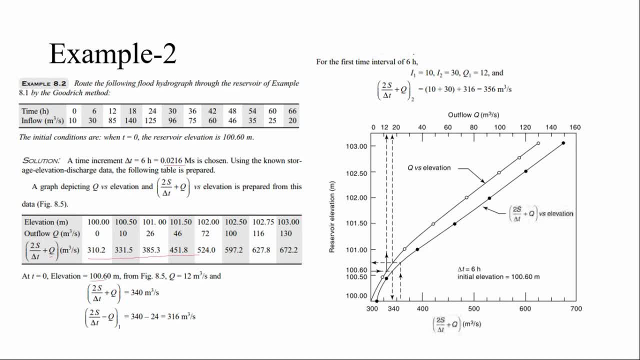 Now what you're doing is initial elevation is 100.60 given. Now I don't have 100.60 here, So what do I do? I need the value of this thing, 2s by delta t minus q. So first I have to get 2s by delta t plus q. 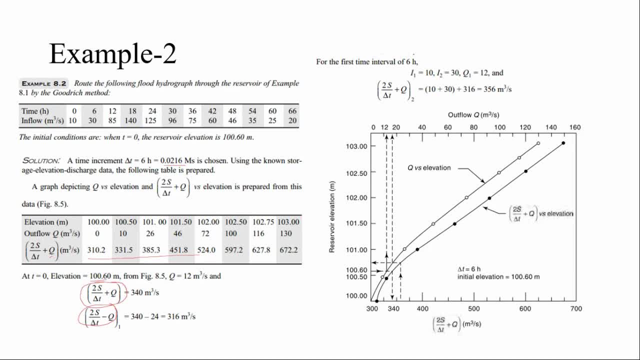 So 2s by delta t plus q, corresponding to 100.60, will be between these two values Between 321 and 350. So it came out to be 340 at interpolation. You can do the interpolation. you'll get something like 340. linear interpolation will work out here. 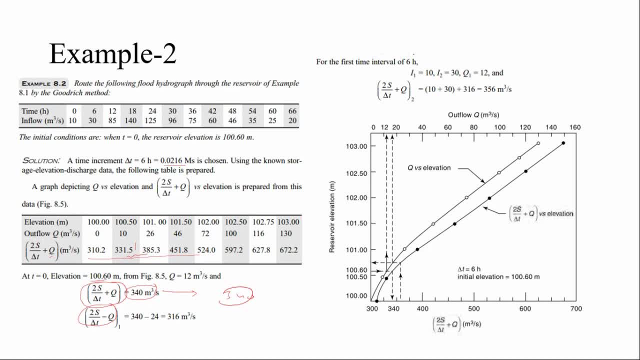 you can also follow any interpolation method. so what is next? once you get this value, simply subtract minus 2q, q is 12, corresponding to this same number. we can also do interpolation: if 10 is equal to 100,, 1 is equal to 26,, then how much is 100.6?? 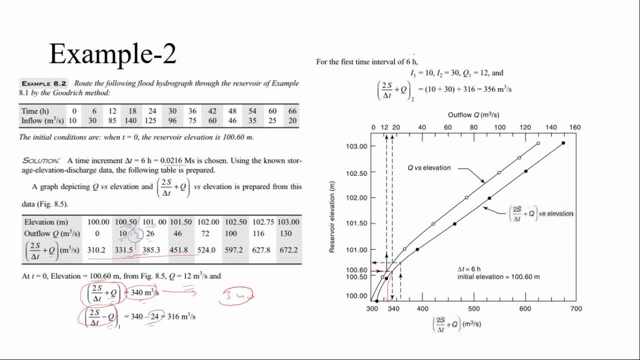 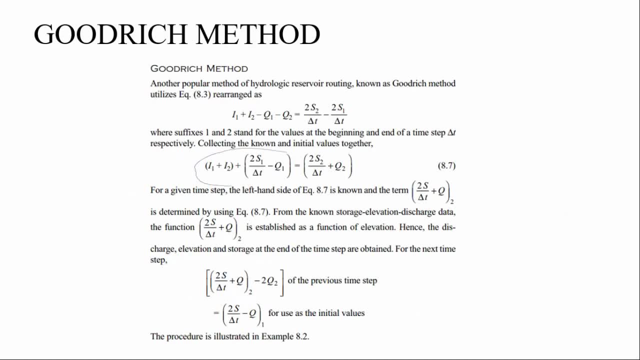 it will be about 12. subtract 12, 2 times, it will be 3.6. we got the first value. now we have the equation, because we are going to use this equation: i1 plus i2 plus the negative value- how much is that? 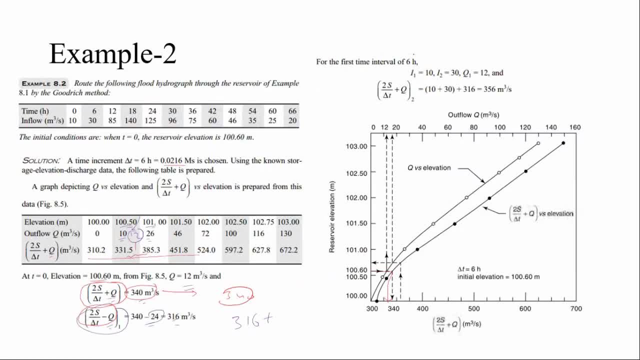 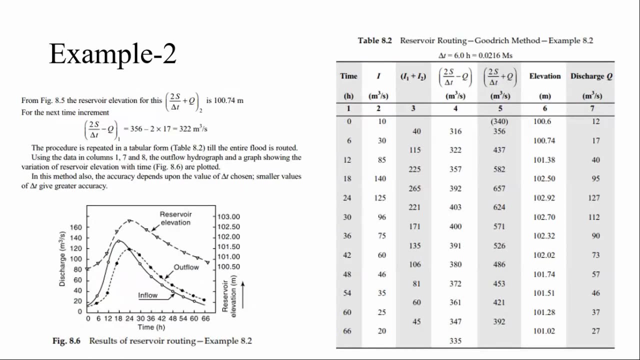 316 plus i1 plus i2, how much is that? what you have is between 10 plus 30 is 40. what do you get? you get 40 plus 316, this is 356. we got the value. the process repeats itself. 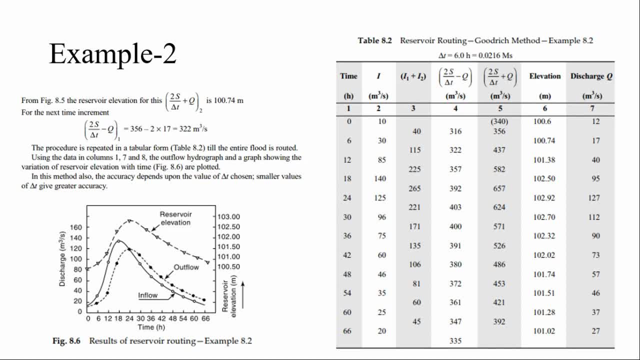 you can get the direction and elevation from that value. see the process here again. time 0 has i given. all these values are given. sum these two. sum these two, get all the相. now how does this quantity look? again, i explain to you how to get 2s minus. 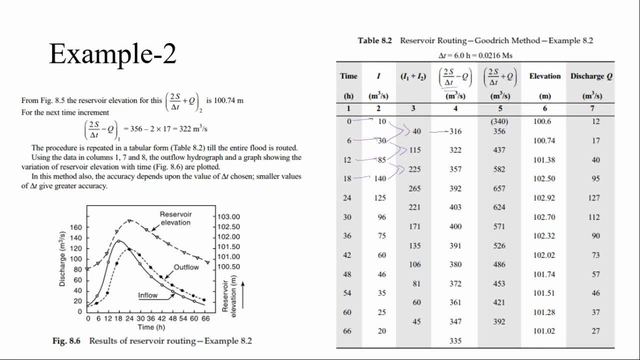 so on initial step we get 316. this is from initial elevation from 100.6, because i was given 100.6. i got discharge from this 100.6. i got this out from these two. so basically i use elevation discharge to find this: quantity 2s by d-q. 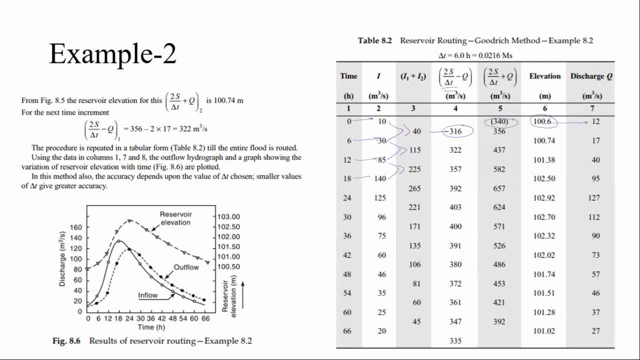 also. this was also calculated. now, once you have this value, just add this up, you get this value. so this is nothing but the addition of these two values. so by adding these, you get this 356. now, from this 356, you can calculate the 100.74. from the 100.74, you will calculate the 17. now, using this 100.74, you will also calculate. 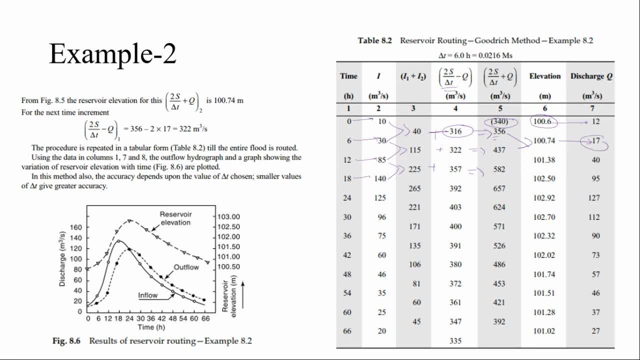 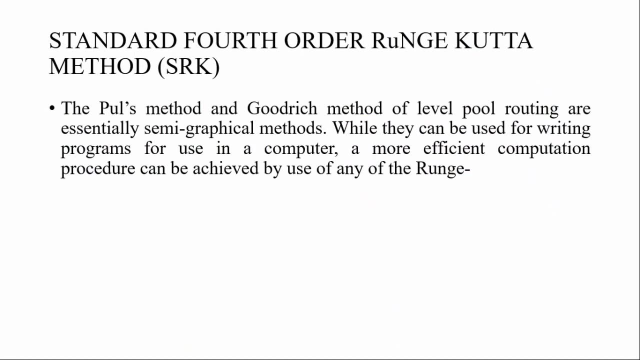 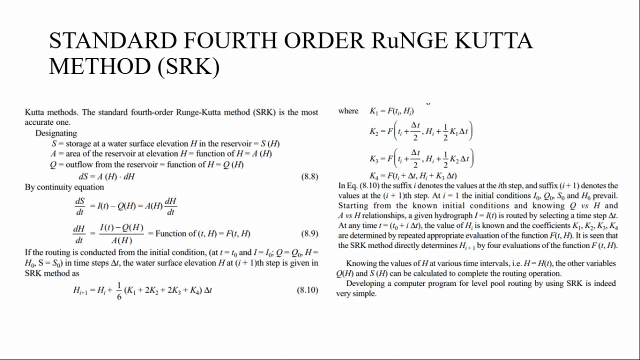 the now using the 17, of course. with the help of this quantity you will calculate: 356 minus 2 times 17, you get 322. 356 minus 2 times 17, you get 322, and this process is repeated, a similar graph you can calculate. then we have a standard fourth order method. so what are those methods? 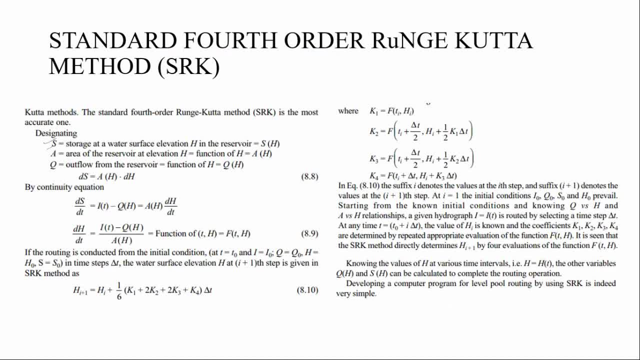 we know s is a storage at a water surface, valuation h. so s is a function of h. we have talked about that. let's say a is the area of the reservoir. it's also a function of height of the area of the reservoir. so we have talked about that. let's say a is the area of the. 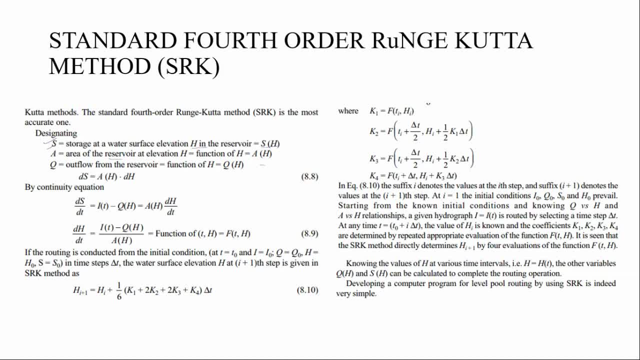 is changing. discharge is a function of height. again, outflow discharge. so if we talk about so, if there is a reservoir in this way, so if we talk about this is its area, so this is the area at any given height into, if you do, is dh, so this dh is basically this dh area. 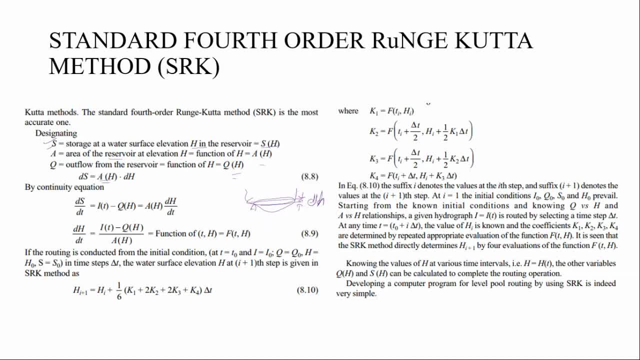 this ds, dh height, if you multiply it with area then you will get an incremental volume. so ds is the incremental volume. now we know the continuity equation is: ds by dt is equals to i minus q, or that is also equals to ih into dh by dt. so by rearranging it you get: 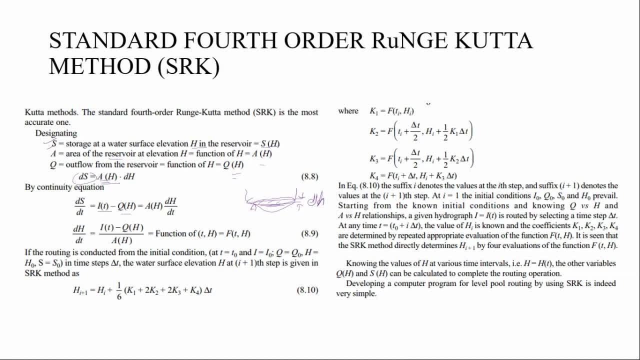 dh by dt equals to i minus q by ah. it's a function of time and h now it's a multi variable differential equation: f model here now rangakutta method. what does it say is: of course you need the initial values. it says that h at any other time step will be h at the previous time step. 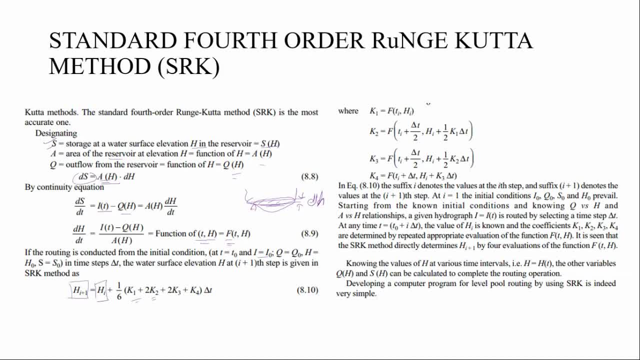 plus one by six: k1 to k2 to k3 and k4 into delta t. now what about k1, k2, k3, k4? k1 is slope at t1. h1, k2 can be calculated with the help of k1 delta t, so x value will be ti plus delta. 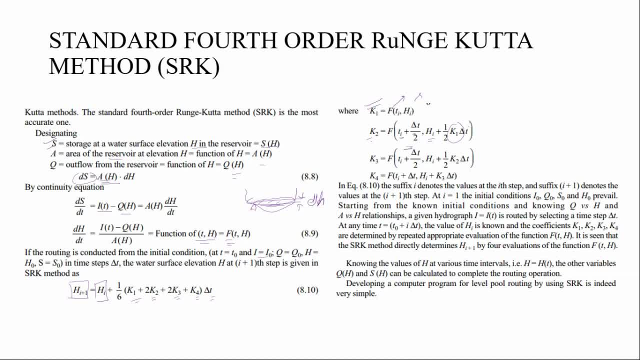 t by half k2 and k3. x value will remain the same. difference in h value will be y k value difference that will be hi plus half k1 delta t, hi plus half k2 delta t and k4 is finally ắn, this internet rk made up of four methods, because you are using up to four, so you can. 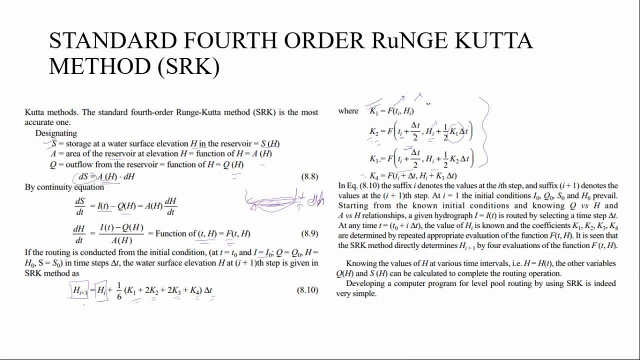 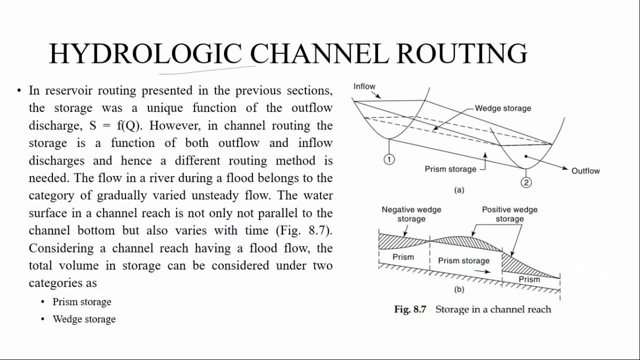 employ this to get the h i plus one. so you can also expect some portion on this rk method. now we look for some hydrologic channel routing. so surface, so its a difference, the channel routing or its melt. so in channel routing there is a causal linefasting di. until then here we Are going to use internal chronological, so for for thermalichts, here you can君usey this here in this. So now we are going to go and test a question. Now there is a basic Wonder, so almost to say that underrin schöwas the reaction which we take that area, but it worked. 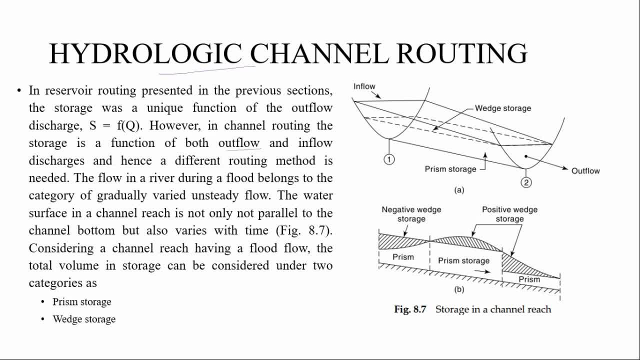 storage is a function of both outflow and inflow, so both have a function and has a different routing. so in channel routing we don't use outflow in reservoir, but in channel outflow is used somewhere. that's why throughout it's a function of outflow. 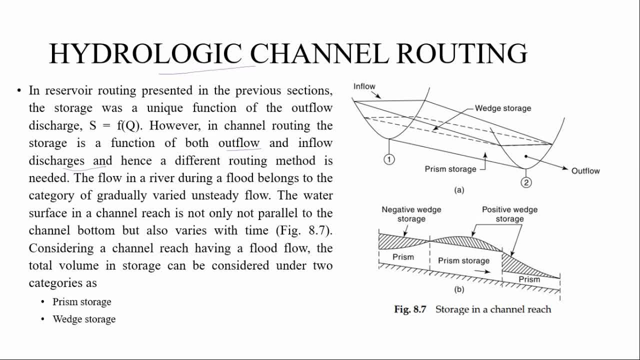 outflow has to be changed. if you consider channel, then it can be divided into two parts. one is the prism storage. if i draw it in parallel line with this channel, then this area looks like a prism. if it was a triangle then it would be a triangular prism. 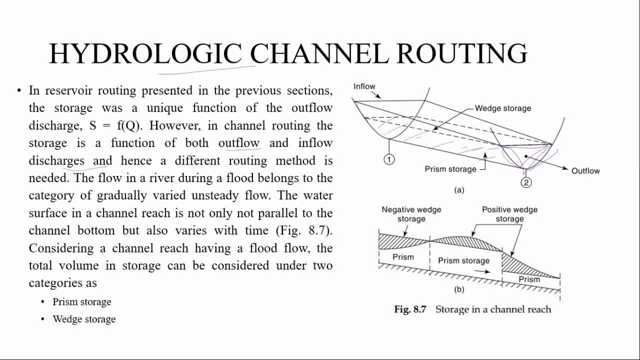 and the volume would be below it. then the upper one can be a wedge, this triangular shape. so this whole volume, this upper one, is our wedge. for example, suppose this is my wave shape. suppose i pick up this section. this is the height of the section if i go backwards. 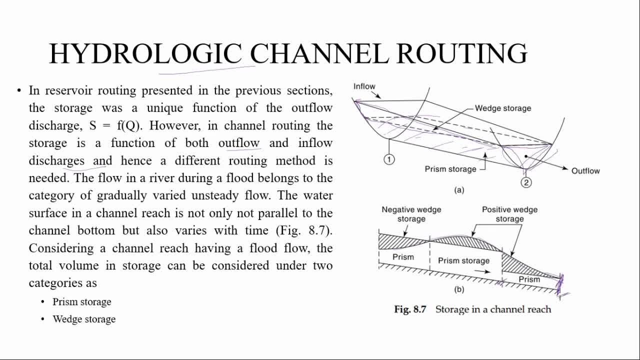 i have chosen this particular section for the routing. i am standing here, i go backwards to this section. once i reach here, i know the water is everywhere clear. so this is the volume of water. now i know this is the shape of the surface. this is also positive volume. 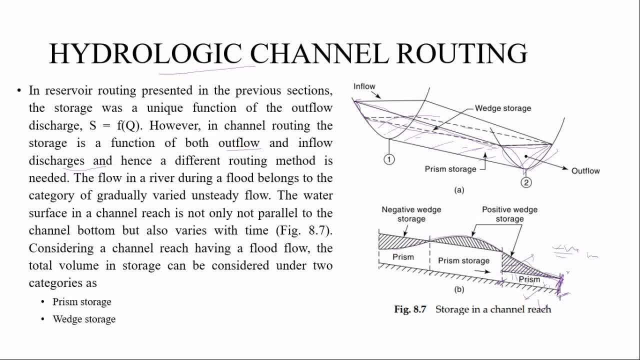 so positive volume of the wedge and positive volume of the prism. so this is my total volume. so this is sum of prism volume and the wedge volume. then when you reach here- i went backwards from here- i found out that if i cut this section there are two volumes. 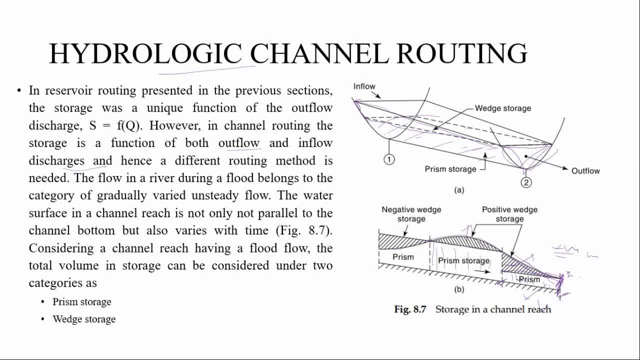 this is prism storage and this is wedge storage. then i went backwards from here. i found out that the surface elevation is like this: now what will happen here? this is my prism storage, but the wedge storage will be negative. so it is a sum of either prism storage and wedge storage. 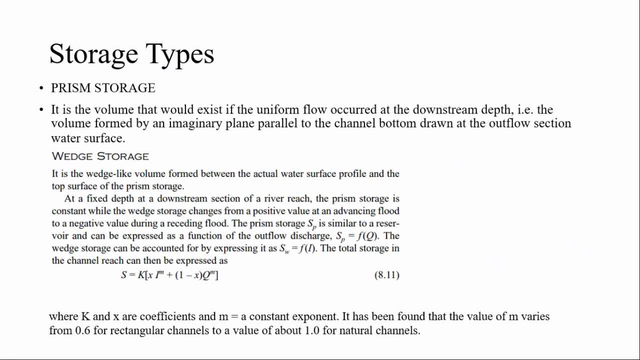 i have explained about this thing. so overall general equation. there are some general equations in the channel. that is k constant, x is another constant and 1-x is 1-x. so i is the inflow hydrograph and q is the outflow and m is the coefficient. 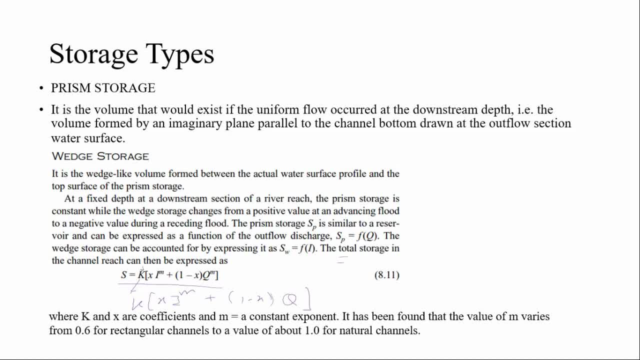 so this is a simple equation: k constant, x is also a constant and im so with kx and m. this equation x basically gives the weightage of inflow hydrograph as compared to the outflow hydrograph. so usually the value of m is changed between 0.6. 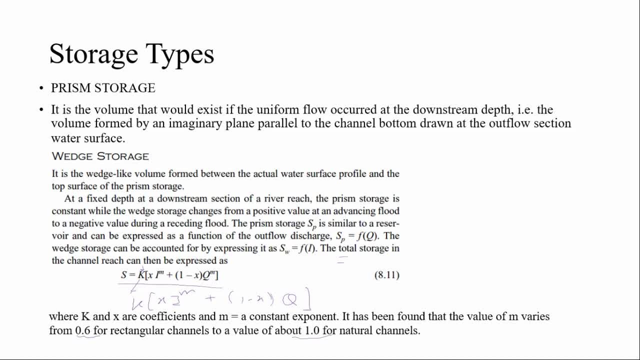 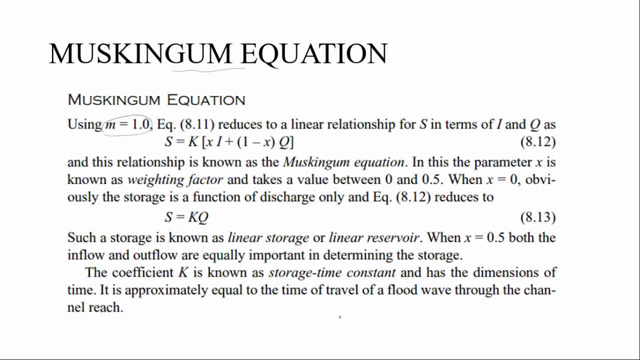 and c1. now, muskingum is an expression method for routing wherein we use m for simplification, so it will be like xi plus 1 minus xq. this is the muskingum equation. x here, as i said, is the weighing factor, varying between 0 to 0.5. 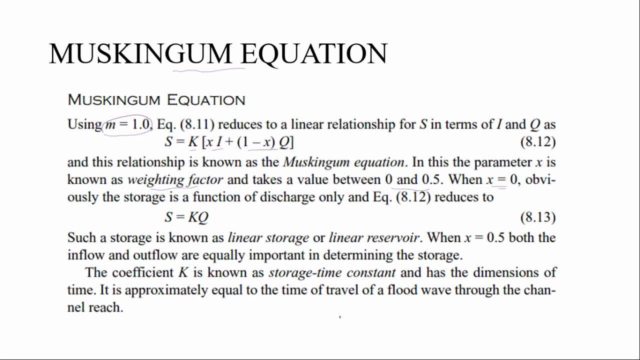 so when x is 0, the storage is a function of discharge only. so why? because if x is 0, then this will run, so this will just become a constant value. if 0 is 1, then q is there, so this will be as equal to qkq. 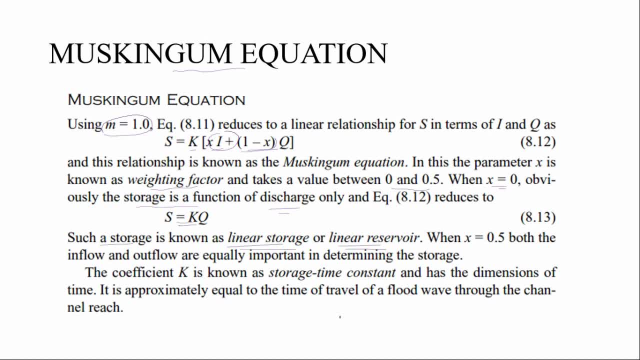 this is called as linear storage or linear reservoir. such a storage is known as linear storage. if 0.5 is there, then it will be equally important. k is called the storage time constant as a dimension of time, volume, discharge of time. how do you estimate this? k and x? 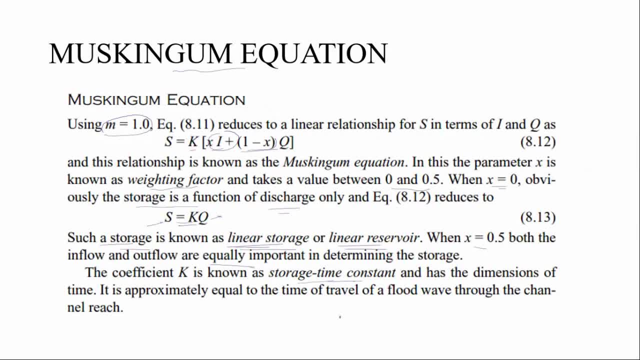 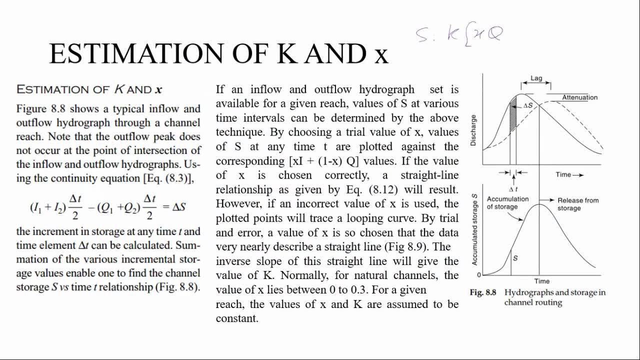 simple method. we have this: s equals to this k into xq. sorry, k is equals to x into i, plus 1 minus x into q. so if you see carefully, if k is a slope, and so what i mean to say is this: s is a linear function of. 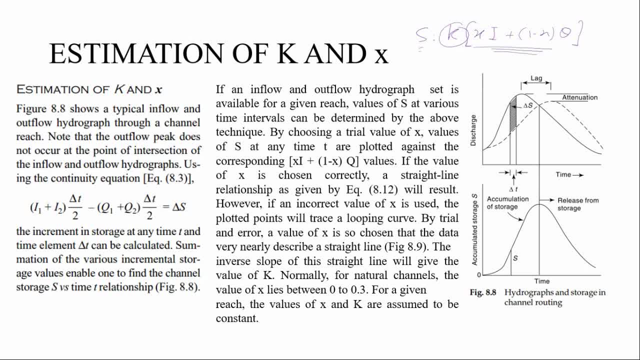 this particular thing with k as a slope. so what do we do is inflow and outflow hydrograph. let's say, for each of our passments i have all the values of i and q, so by that way we can determine the value of x and k. 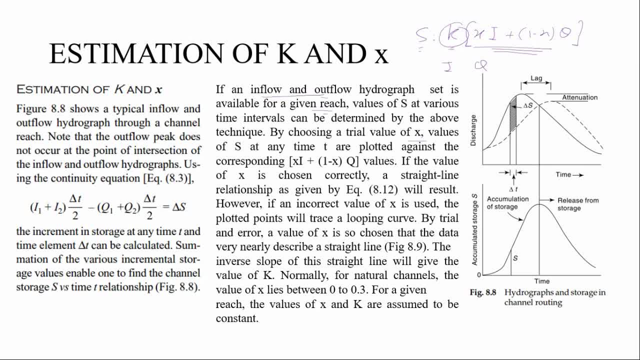 so we choose a value of x, we choose a value of x, then what you do is you calculate these entities, x, i plus 1 minus x, into q, because once you have chosen x, i is known to you, so this entire quantity you can estimate s is also known to you. 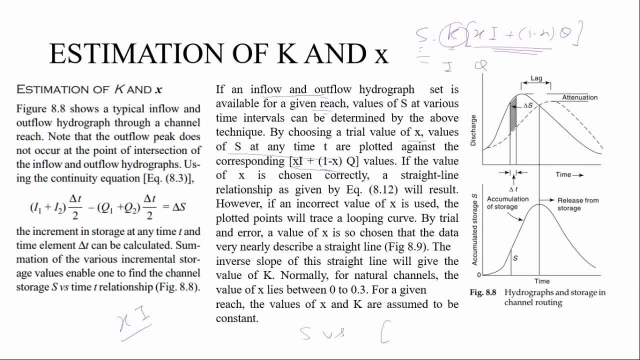 storage is also known to you, then what you do is you plot s versus this entire quantity x- i plus 1 minus x- into q for a chosen x. when you plot it, you want it to be a straight line, because k is a slope and it has to be a straight line. 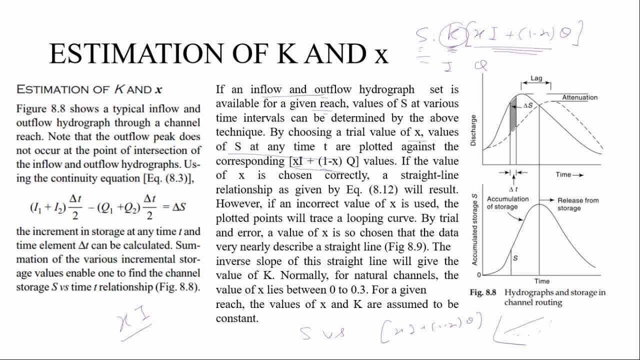 however, if it is not a straight line, it will be varying. so you just keep on trying until you get such a x value so that the data lies in a straight line. so that's how you get the value of k index. i will give an example by saying: 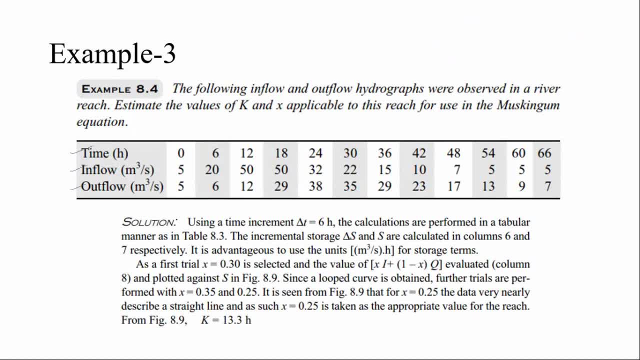 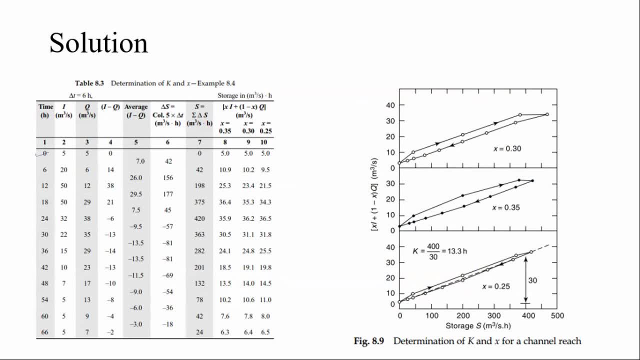 time, inflow and outflow given m. so let's just go directly to the table form. so for different time intervals you have inflow and outflow. so what you want to calculate is x times i plus 1 minus x times q. now storage is nothing but. 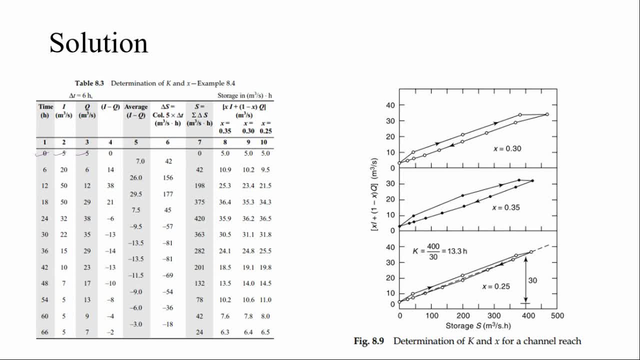 the difference of your i and q. so what you have is i minus q for each section average value from these two. you can calculate the average value. multiply it by delta, t, time step, 6 hours, you get this. 42 times 56 is a product of 6. 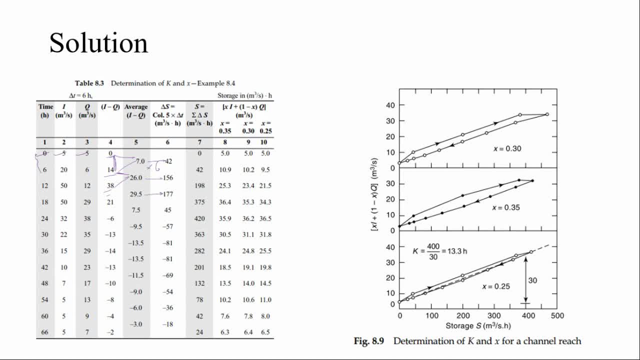 and cumulative storage. you can calculate. keep on adding them. so columns are clear: i given q, given i minus q, 5 minus 6, 20 minus 6, 40, 50 minus 12, they are d8 average of these two average. now, this you have already seen. 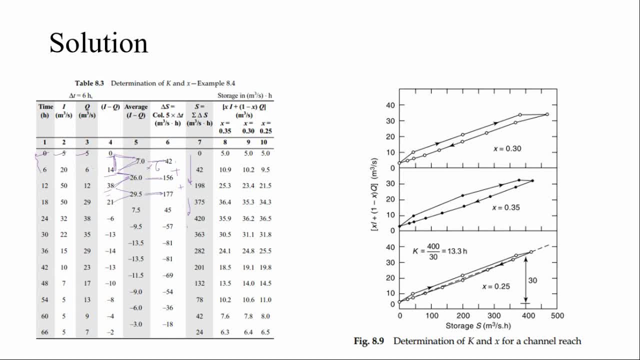 multiply by time, step into 6, into 6, into 6. cumulative at them, you get this value. now, let's say we choose a value of x equals to 0.35. when you choose this value, you calculate this entity: x i plus 1 minus x q. 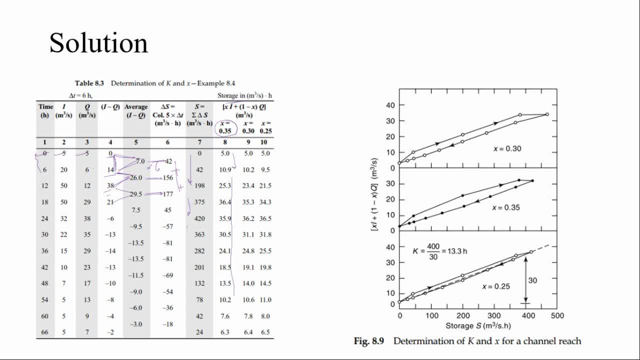 you get all this data. x equals to 0.35. when they plotted this data, they gave something like this: this is not in a straight line. some points are going out. then what they did? they changed the value to 0.3. you can see the curve has changed. 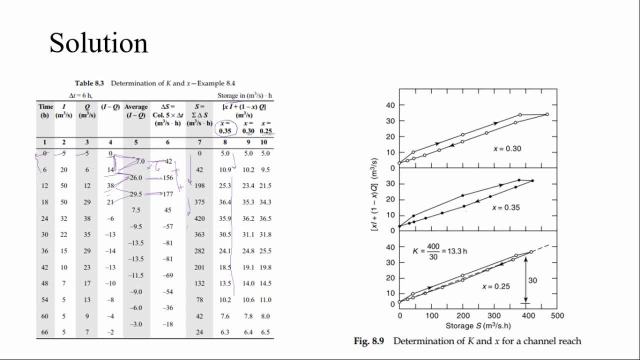 so it required them to change further 0.25. so you can see almost it is in a straight line. so you want to reduce this area of the, this shape, so you want to make it into a straight line. you have found your x value, so this is your x value. 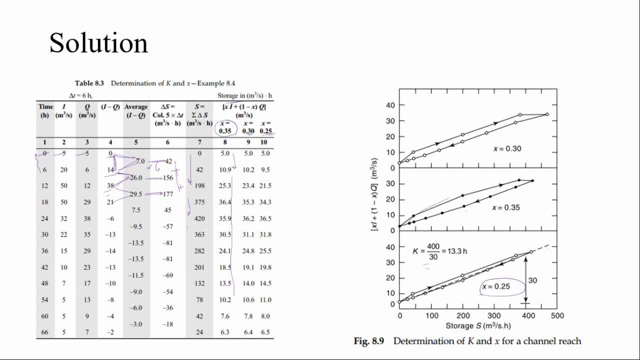 now you can calculate the slope. slope will be nothing but slope of this equation. y equals to mx, so this you get as the fold by 30. this is how you can calculate the slope. so you have to know why i put it up out here. that's why you are seeing it as fold by 30. 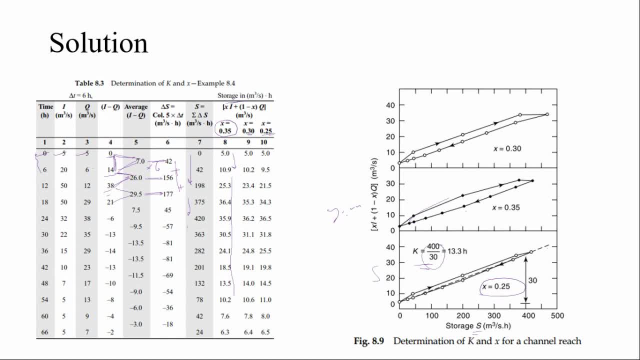 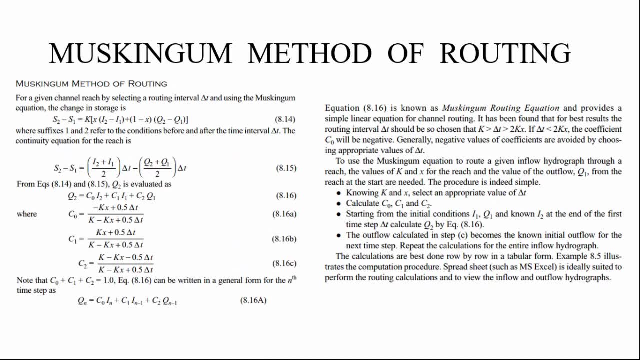 you can have it in any other way. s can be on this axis, this particular thing can be on this axis. that also is possible. now, once you calculate k and x, how do you actually route it? let's see how it works. so this s2 minus s1. 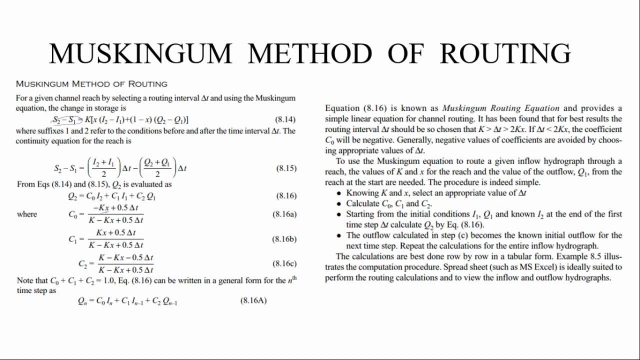 this delta s is nothing but k into x, i2 minus i1 plus 1 minus x, into q2 minus q1. so for delta t time interval, so change in storage is x into change in inflow plus 1 minus x change in outflow. 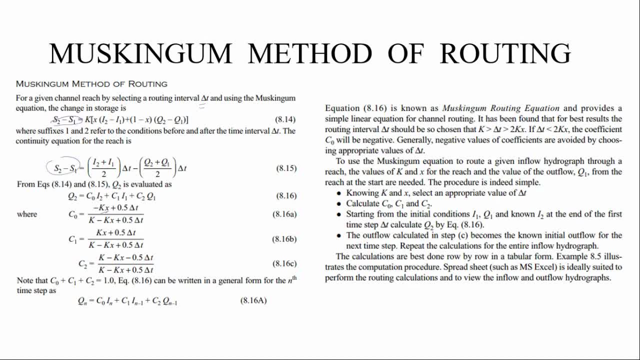 and we also know what is s2 minus s1, average inflow minus average outflow for that delta t time. now, if you see these two equations, they are equal. what is the quantity in this? i1, i2, q1, q2. so basically, q2 has to be a function of 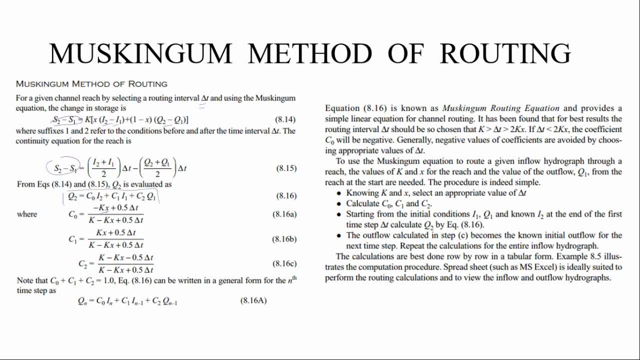 i2, i1 and q1 some coefficients: c0, c1, c2. once you compare these two equations and you equate them, you can get this: here is the value of c2 minus kx plus 0.5 delta t upon k minus kx plus 0.5 delta t. 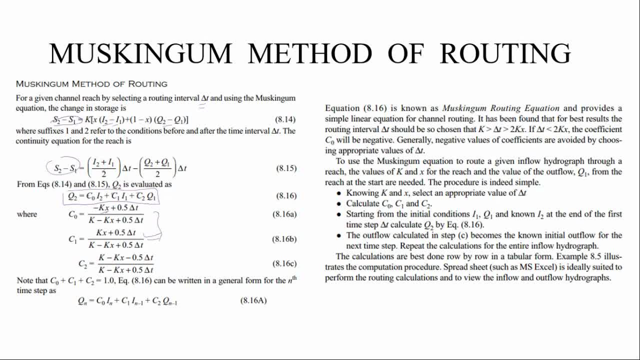 just like that. you have some value of c1. you must remember these values. you must remember these coefficients. they will not be provided to you in exam. so once you have got these values and we may note that c0 plus c1 plus c2 equals to: 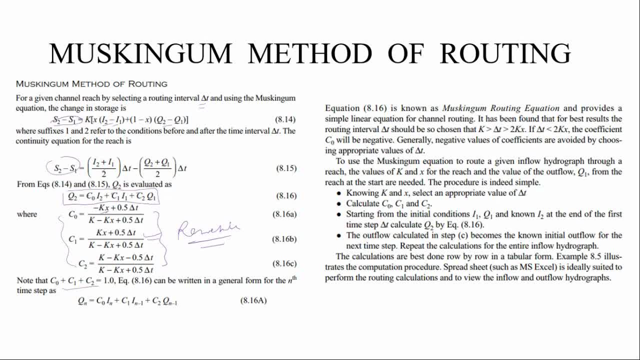 1, so that's why it's a general equation. so qn is c0 in plus c1 in minus 1, so c2 qn minus 1. so this is called muskingum routing equation. one more important thing that you need to remember is: 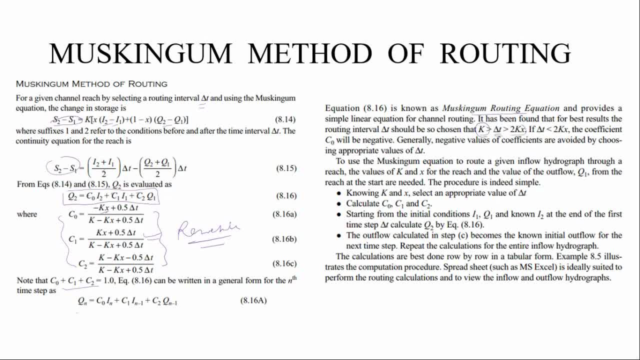 delta t should be smaller than k and should be greater than 2kx, because if 2 is smaller than k, then c0 will be negative, so it will be on the back. we don't want that. so t is so small, its limit is between k and 2kx. 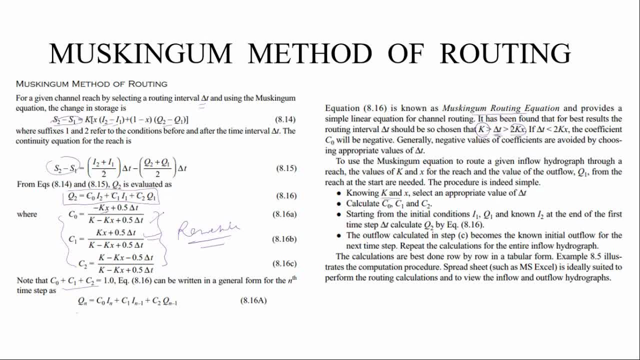 so once you have the step of this, once you have the k and x values, you get an appropriate value. delta t calculate c0, c1 and c2. this will be removed from all this. i1, q1 is given, i2 is given at the end of the time step. 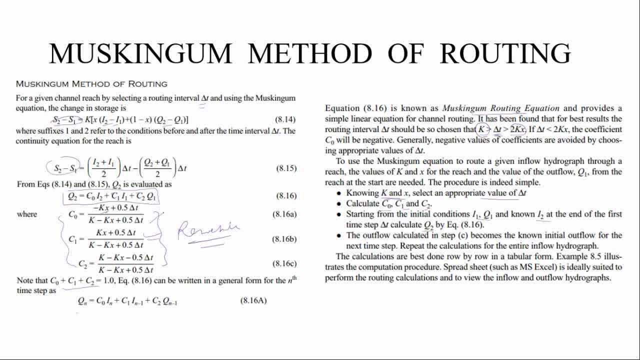 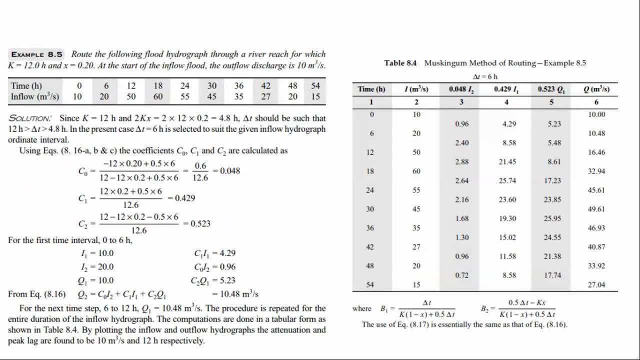 a is always given to you. calculate q2. now q2 has come, so it is next for that. what will be made? q1 will be made. process is repeated. you will get all the q values. same example here: time with inflow is given, k is given 12k, 12 hours. 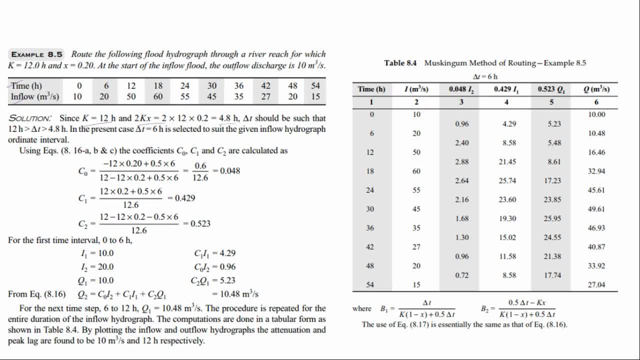 2kx- 4.8 hours. so you have checked 2kx. so delta t should be 12 and 2kx means 4.8. so you have assumed it according to the time step. 6 hours: c0, c1, c2. 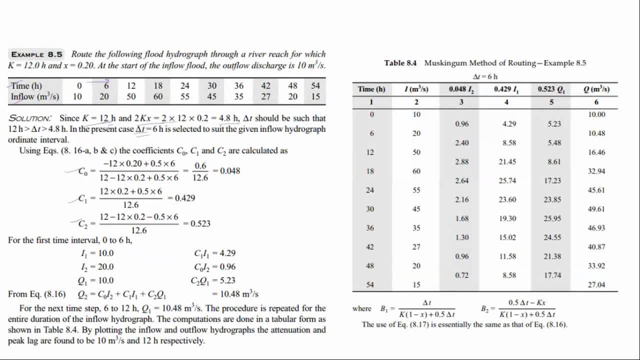 based on the equation, you can calculate c0, c1 and c2. now, i1 is given 10, i2 is given 20, q1 is given, 10 given to you. so c1, i1, c0, i2 and c2. q1 i removed. 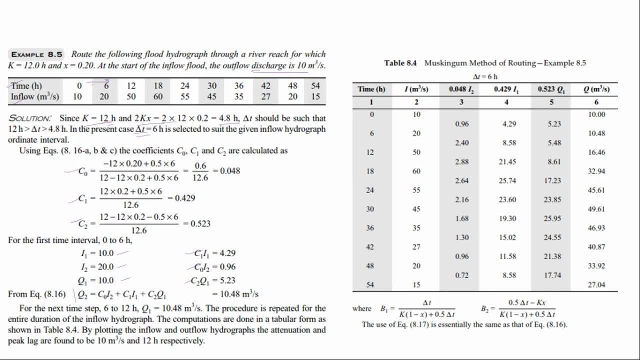 and from that i got q2. simply just multiply this 0.048 with i1, with this i2, c1, 0.429 into your c1 into i1 and c2 into q1. add all these three terms, you get this 10.48. 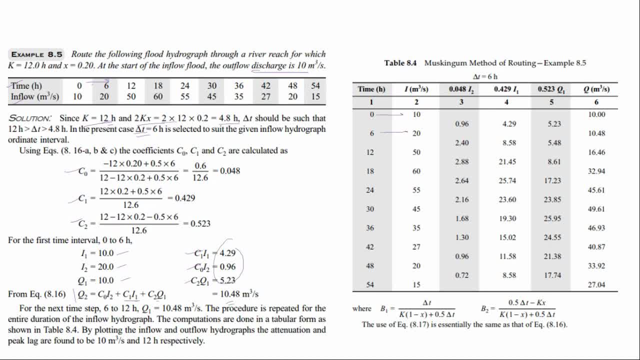 see the table of all the information is given. so 0.048 is your c0, 0.429 is c1 and 0.523 is your c2. square 2c multiplied by square 1 is equal to q1- c1, so you get this value of. 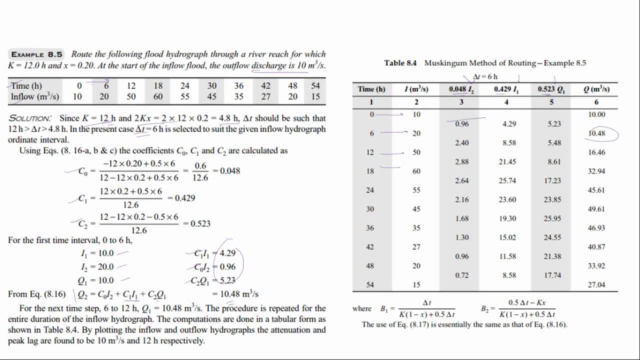 10.48 for this particular time step after 6 hours. now this quantity here becomes your q, now i1, i2, we all know. when i came to this step i knew i1, so in this i can calculate. now, for this step i need q1. the new q1 becomes my. 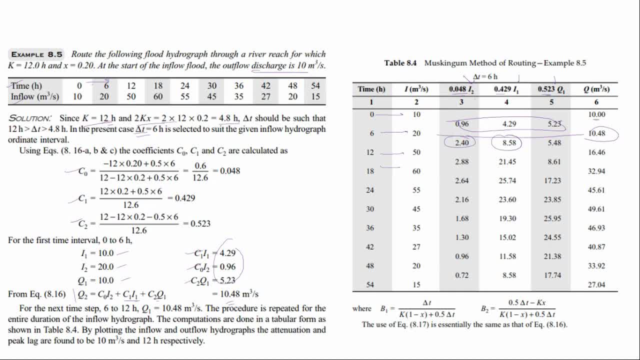 10.48. so instead of 10 for this step now i will use 10.48, so i get 5.48. when i product it by 0.523, 5.523, i get 8.61. the process is repeated for the all the time steps. 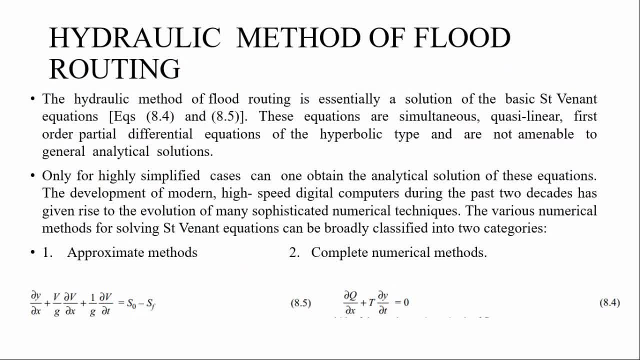 then there are some hydraulic methods of routing. as i said, there is a continuity and momentum equations, so these can be used using some computer numerical methods, finite element method. so they are not related to your course, so for now, but they can be used for computer modelling or 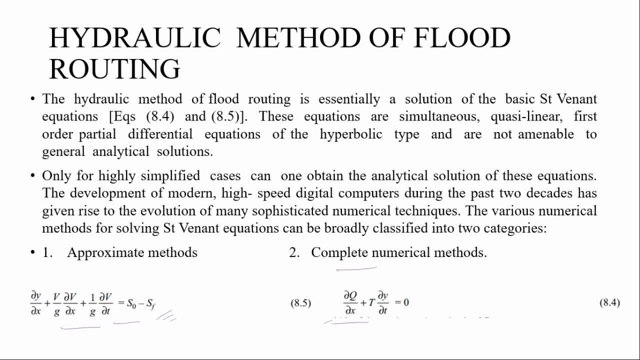 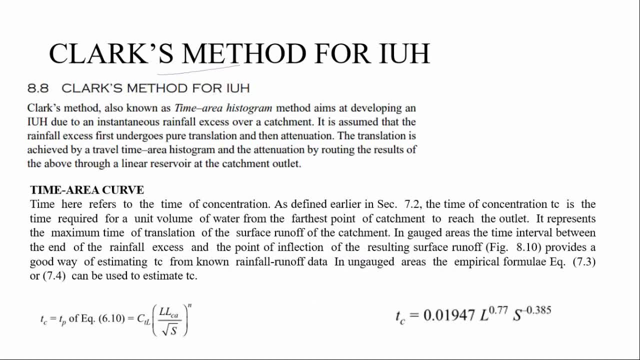 hydraulic modelling. they are difficult to solve analytically. that's why we use those simulation models. then there is a Clark's method using the instantaneous unit hydrograph method. so what do we do in this? so Clark was the person who developed the IOH. due to instantaneous 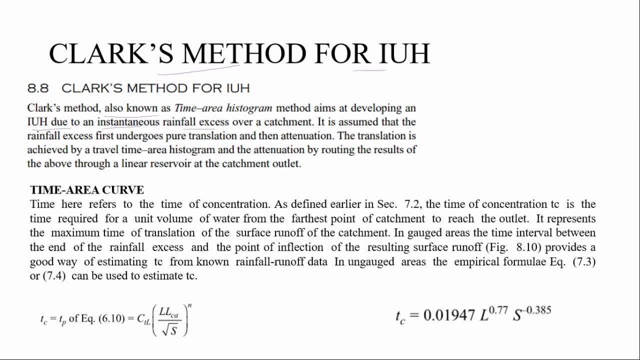 rainfall axis over a catchment. so in this term the important term is time of concentration. that should be known. so time of concentration is nothing but a constant. L, LCA root S, power N- again, i have discussed it earlier. also, L is the length of the basin. 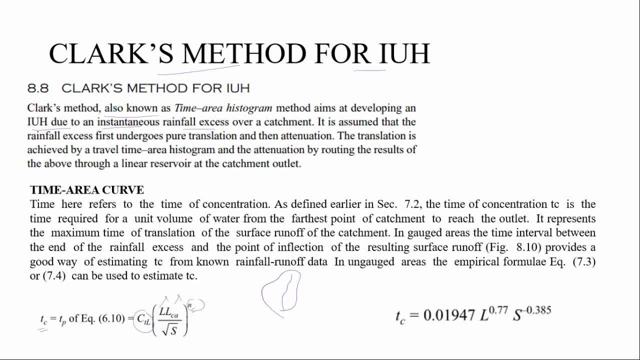 the main channel of the basin. L is the length of the main channel and LCA is along the main channel but near the centroid, S is the slope of the channel. we can't get it from this length or slope, so in either way, you just need a value of 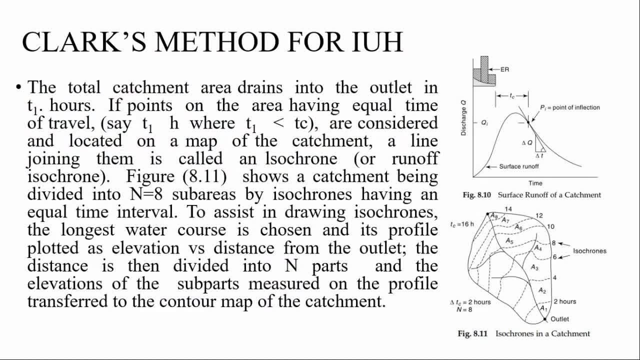 the length of the basin. what to do? i have a basin. i divide this basin in various isochromes, isochromes, isochromes line is joining equal times. so let's say this is an isochrome of 2 hours and this is an isochrome of 4 hours. 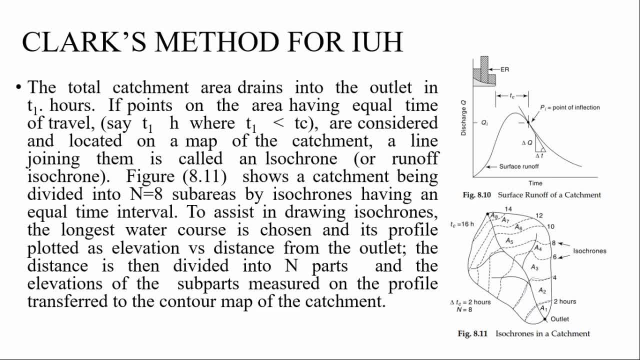 now in what sense. i am talking about these chromes, so this is their time of concentration. means if a water drop falls on this line, it takes 2 hours to get out. if a water drop falls on this line, it takes 4 hours to get out. 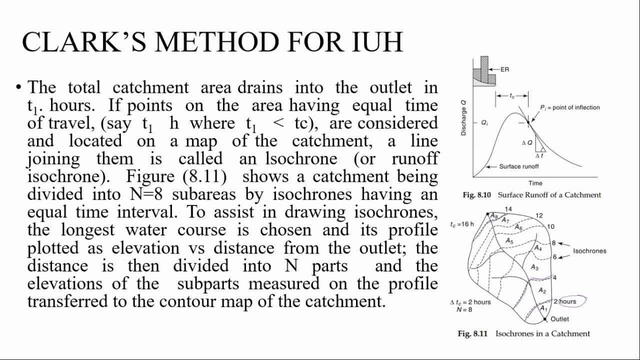 just like that. if a drop falls on this line, it will take 14 hours to get out, so i covered the whole area. finally, i have Tc delta. Tc is 2 hours because area is 8 hours, so whatever water falls on this area, i will get it from 16 hours. 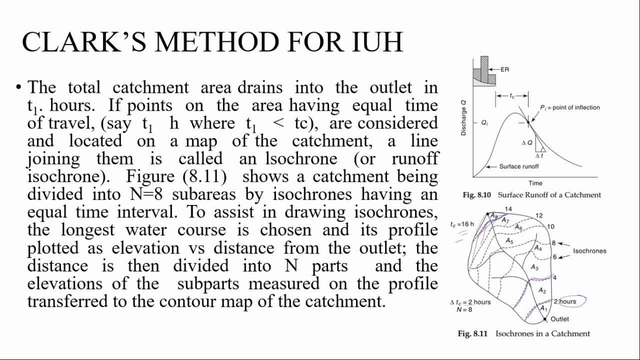 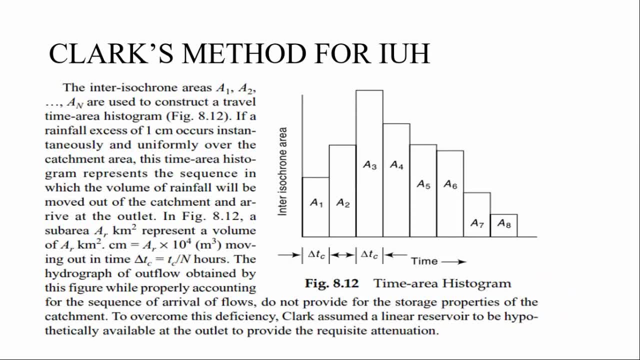 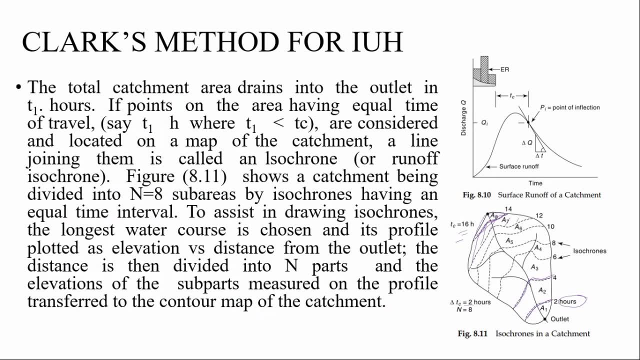 because it is farthest then the water which falls on this area. i will get it from 14 hours. is it clear now? so we have divided delta Tc by Tc. so for different delta Tc we have taken out the area. what will i get from this? 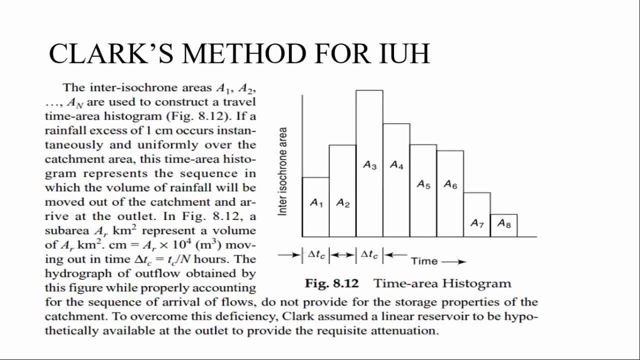 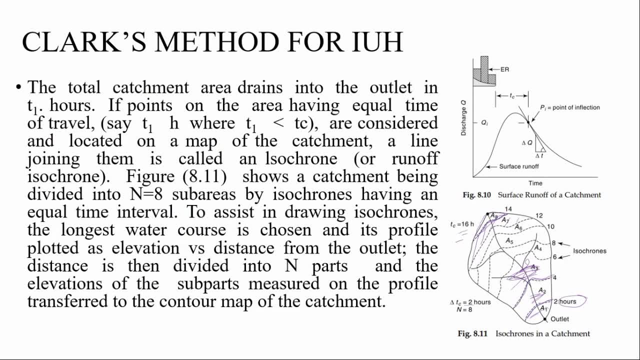 area 1,, area 2,, area 3 and, like that, area 1,, area 2, largest, area 3, area 3 is the largest. so, and this is one more thing i want to mention here, this is, let's say, your hydrograph. 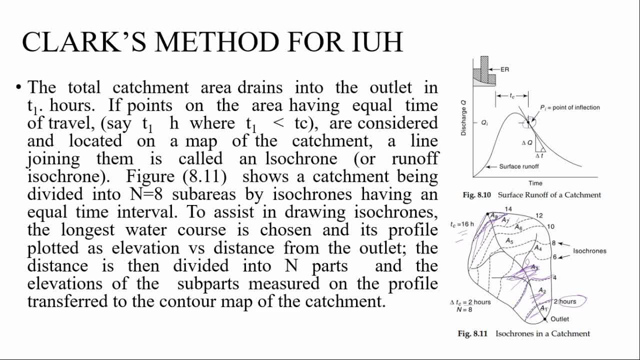 and this is called the point of inflection. this point of inflection is that point when Tc is finished, after that time of concentration is also run, so after that the flow will be less, because all the water has come in this point now, from this point. 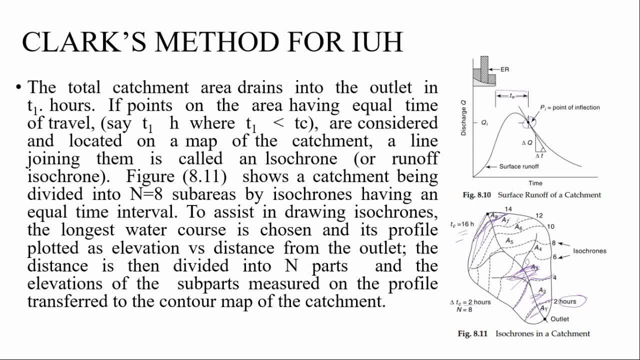 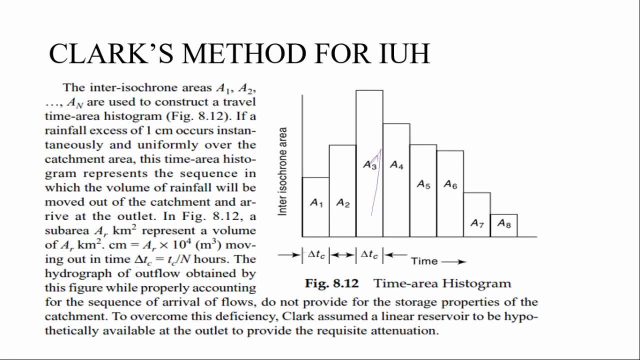 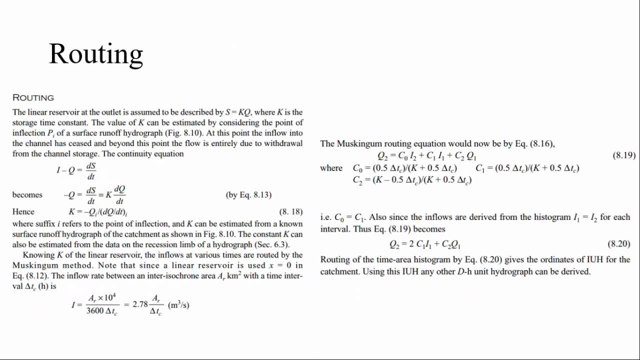 water is coming from the whole basin, so this is a free flowing curve. you can see the use of this. so Ar is the Ar, and A1,, A2, A3. these are the areas for different time periods. now, how does this method work? so, first of all, what we do. 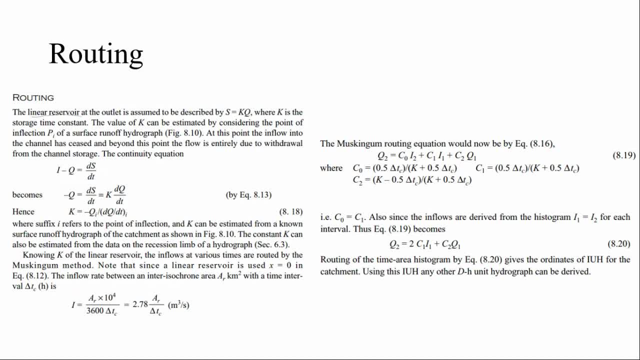 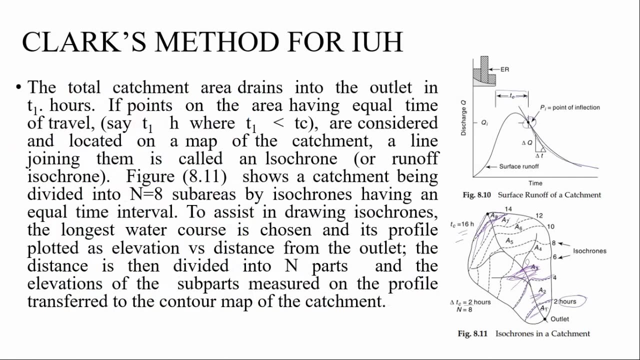 assumption of the clock method is that when we talk about the linear reservoir, we will use that S is a function of K into Q. K is the storage time constant and what is the method to estimate K1? so what we do? we pick up the point like this point: 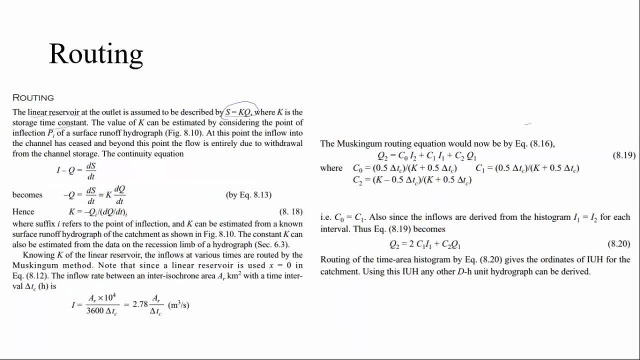 point of inflection. when i pick up the point here, the inflow is stopped, 0, only the outflow is there. so minus Q equals to ds by dt. if we talk about this, S is a function of K, so this becomes: minus Q equals to K dq by dt. 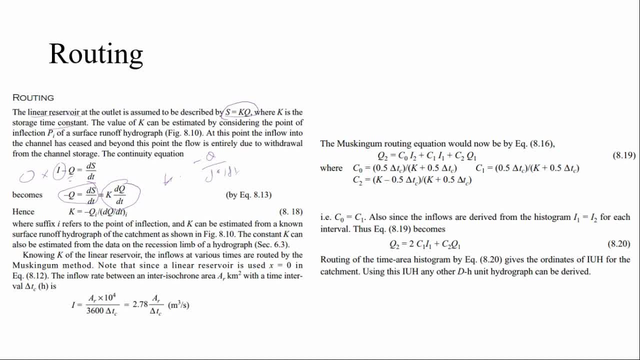 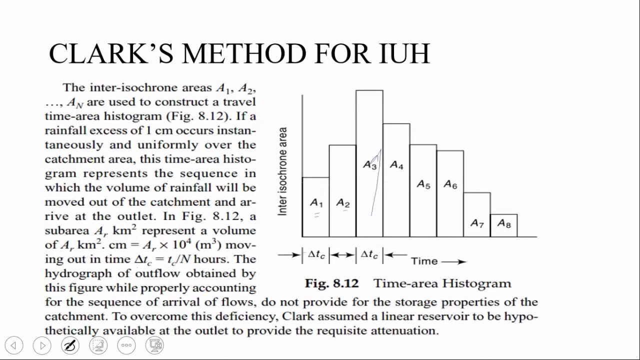 so from here K will be minus Q over dq by dt. in this equation we got K of the point of inflection, so K can be estimated from a known surface run of hydrograph of the catchment S only in any previous hydrograph. if you see its feature. 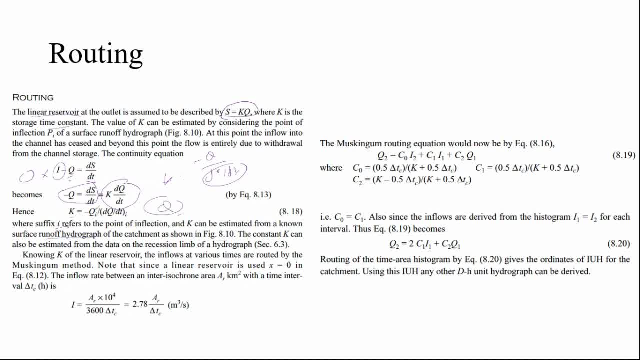 then, with this feature, i can estimate the value of K, because this is a characteristic feature equation. so i can get this basic feature K. now, once i know the value of K, because its a linear reservoir, now i can go into my method, that is, the musking method. 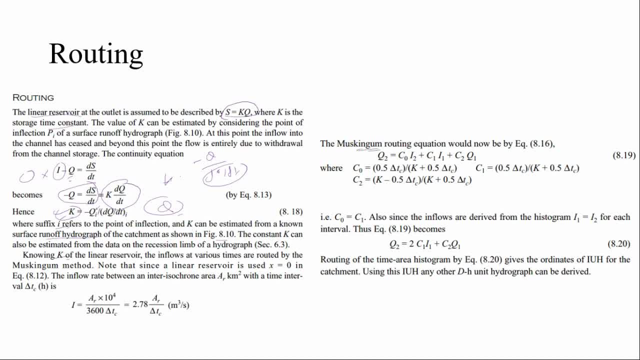 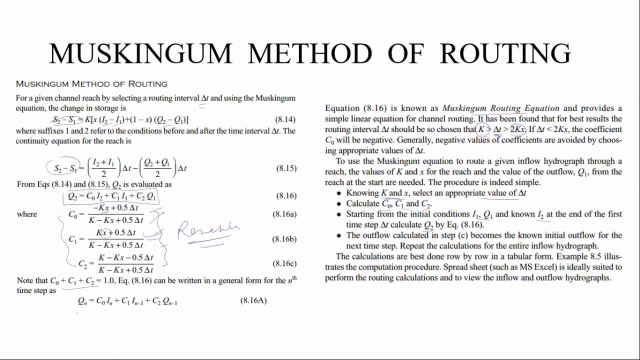 now i can use the musking method for the average value. now one more thing: since i am using a linear reservoir, X will be 0. now we have seen that. so what is the meaning of X0 in this equation? X will be 0. so the formula of constraints. 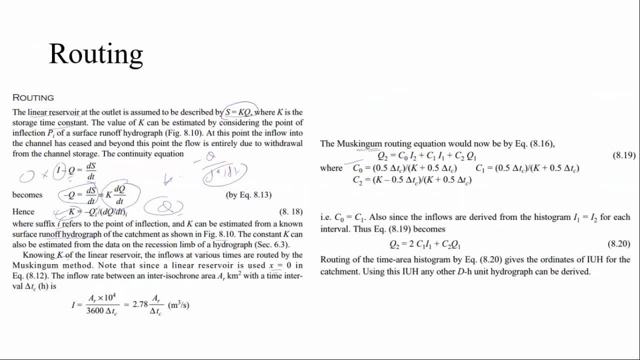 will change a little. C0, C1, C2- there is no role of X. and one more thing is that the inflow rate between the area AR and time of concentration Tc is. this is the inflow rate, so this you can estimate. so, area divided by time of concentration. 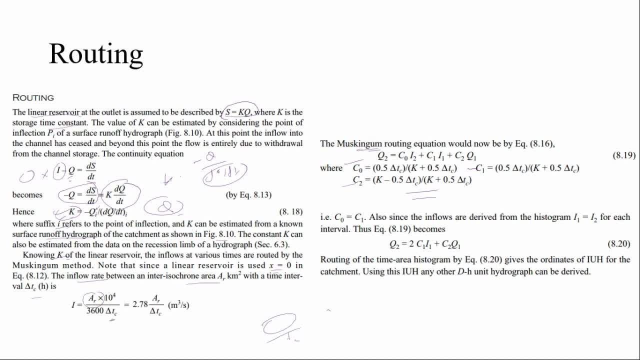 what will i get? inflow rate is it clear, in meter cube per second. so to get it into this area, converted to km2. so all these factors are used to convert to m2 per second. so you get this equation. so how much inflow is getting? 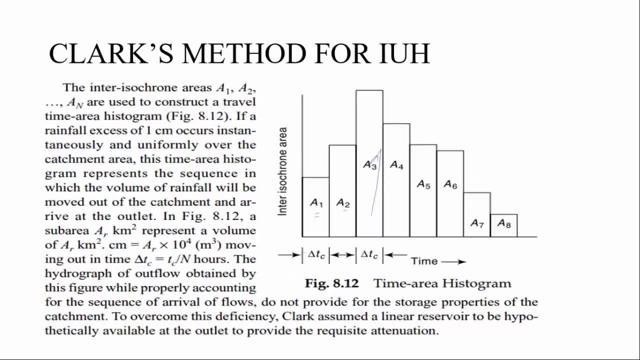 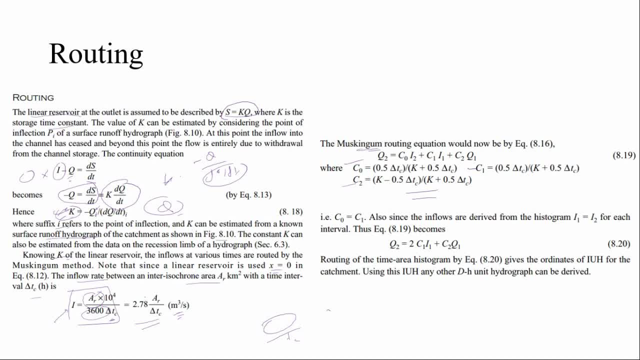 from this particular areas. now, once you have the value of K, known value of K, you can get value of I. so different area, different delta, tc. you can take out i so you can use this equation: q2 equals to 2c1, i1 plus c2. 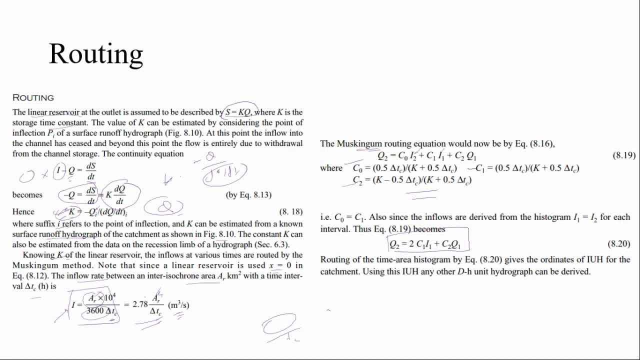 q, i2, i1, q1, because in this equation, see what we are getting: c0 and c1 are equal because x is squared, so it will be 2c1- i1. there will be some difference here. now let's see an example here. 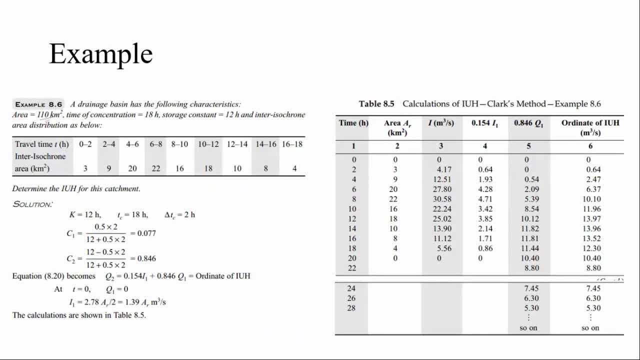 in a machine whose total area is 1 and 10, we have time of constant 18 hours storage, coefficient, 12 hours. this is your k value. isochrome is given for 0 to 2 hours. area is 3, so a1, a2, a3. this is given for different different. 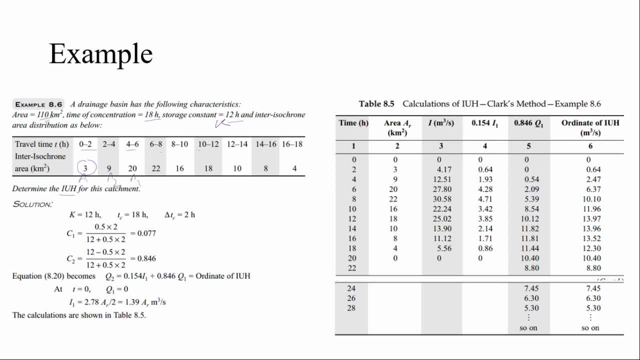 time intervals we have to make its iuh. iuh is basically outflow discharge, but instantaneous, alright. so k is 12, 12 hours, tc given is 18, 18 hours, tc is 18 hours. so delta tc is how many sections: 2, 3, 4, 5, 6, 7, 8, 9, 9, 18 by 9. so i got 2 hours. 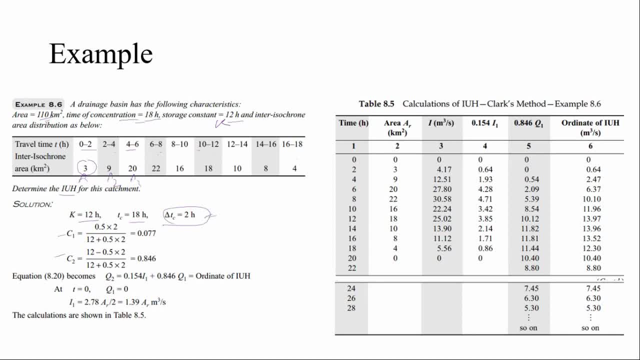 so i can take out c1 and c2, because c0 equals to c1, so it is not required in this formula. so i have this. so what will be my q2? it will be 2 times c1, i1 plus c2, q1, 2 times. 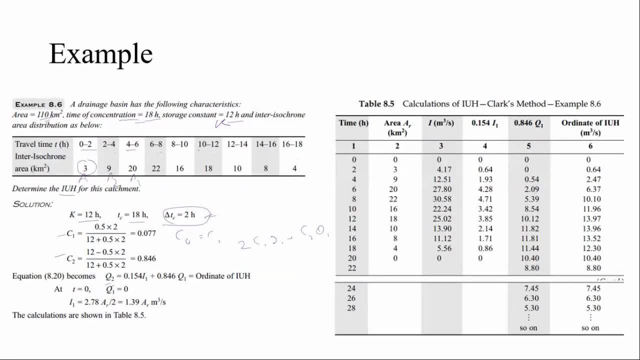 c1 i1 plus c2 q1, now at t equals to 0. initial time is 0. at initial time: 0, 0, i0. this 0, this 0. now, as you are in time interval 2 till this 2 hours, which area is contributing? 3 km square area? 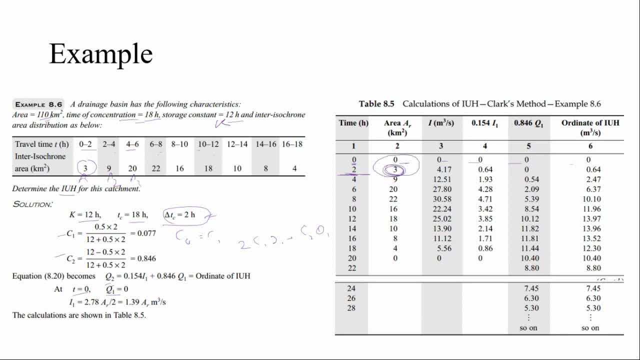 is contributing. ok, that's fine. how much inflow is coming from that particular area? so that is the inflow: 2.78 ar upon 2, 2.78 into ar is your 3 divided by 2. this comes out to be 4.17. 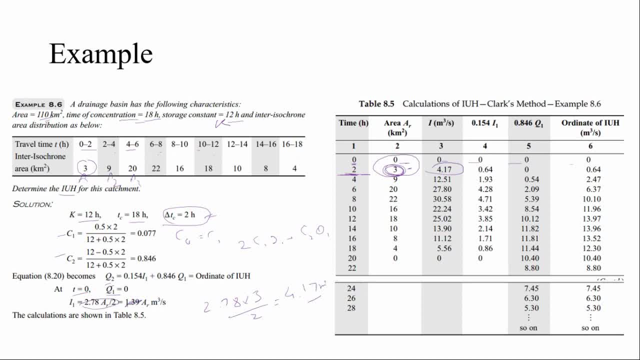 4.17 meter cube per second. you are getting this value multiplied by 0.154, as the demand of the equation q1 is also 0, so there is no outflow. we will get 0.64 to 0.64. sorry, not this one. 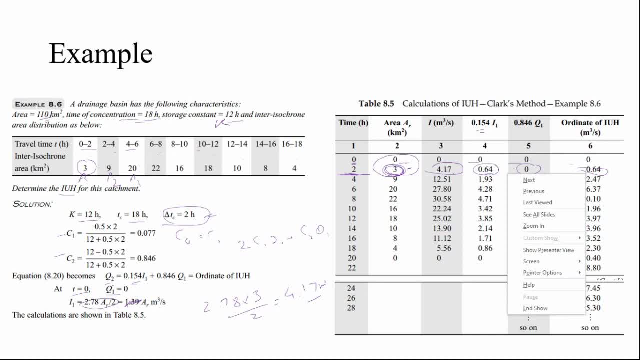 we will get 0.64. now i have to make q. now i will come to step time interval 4. sorry, if i come to step 4 then the area contributing is 9 hours. now you can check that when you do this: 2.78. 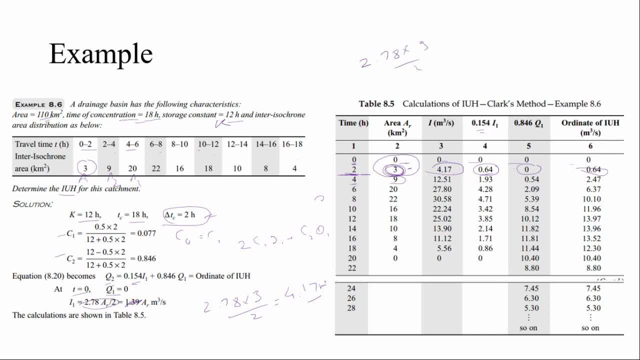 into 9 divided by 2, 2.78 into 9 divided by 2, you get 12.55. this is the area contributing between 2 and 4. now multiplied by 1.54, i1. now this previous time, step 0.846 into q1. 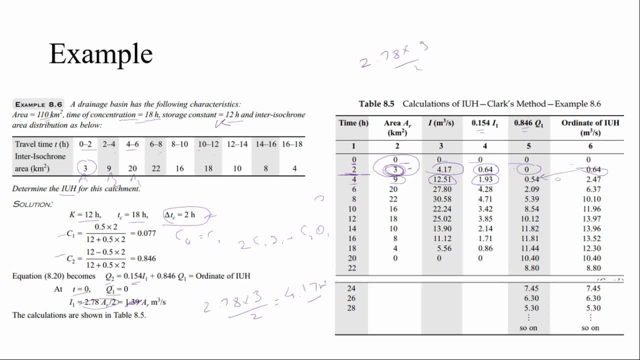 was there. if you multiply by 0.846, you get this value. add on these two values, you get 2.47, and this process is repeated till your time is ended. this is infinite process. that just goes on, alright. after 10.40. after that: 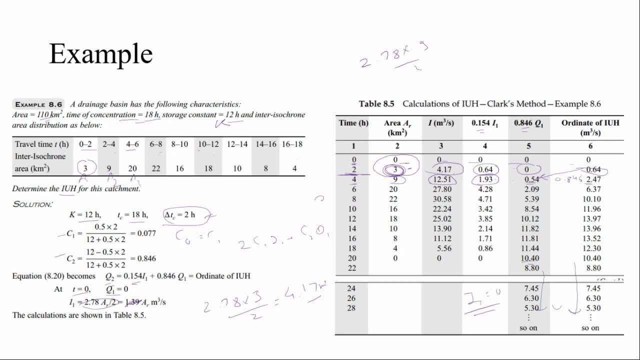 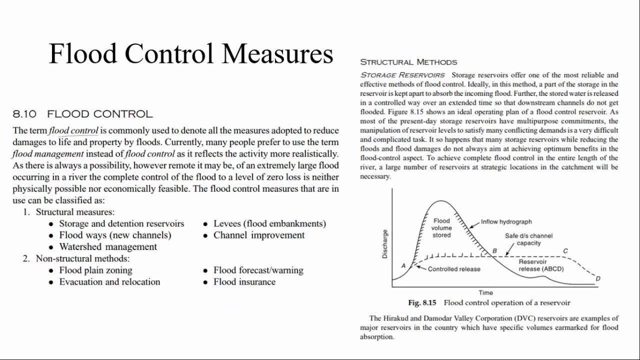 inflow is finished. i is 0 now. ok, this is all about the flood routing things. now we will discuss some of the flood control measures. flood control is a commonly used term to denote all the measures adopted to reduce changes to, to reduce changes to life and property of floods. 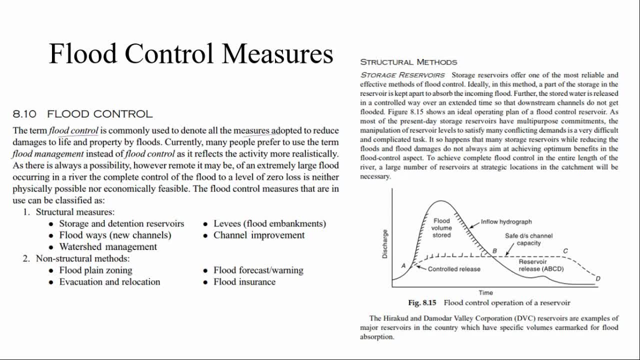 so mostly we use flood management term instead of flood control. number of methods are structural method: storage, flood management, reservoir levees, floodways, channel improvements. so these all are the. so these are the various structural measures we will discuss one by one each of these. so, storage reservoirs. 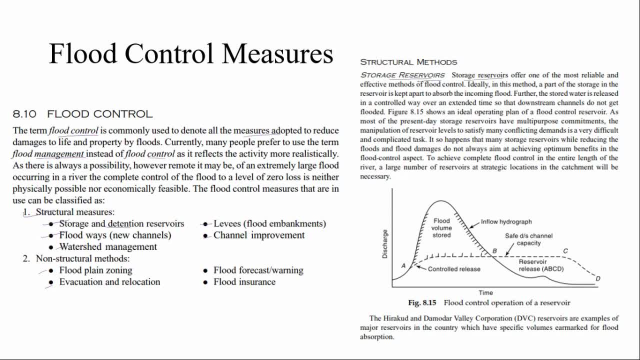 so storage reservoir. normally we make land reservoir. it is one of the most reliable and effective method of flood control. in this method, a part of the storage reservoir is kept apart to absorb the incoming flood. a large part of the water is stored like this. we used to get flood like this. 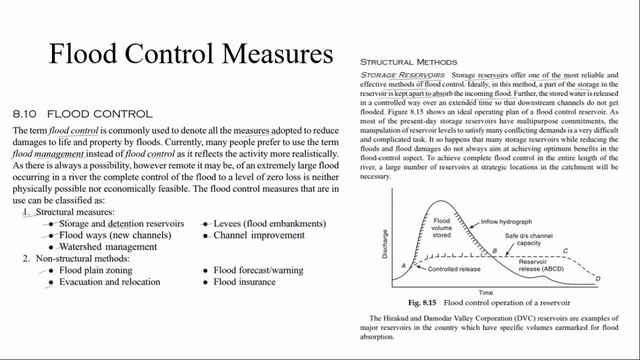 we did not give this reservoir, so all the water that came we stored it here. now, when the water runs, we can release it. so in constant flow we can release it, although naturally it is like this, it is a simple thing. you all know that the stored water release in controlled way. 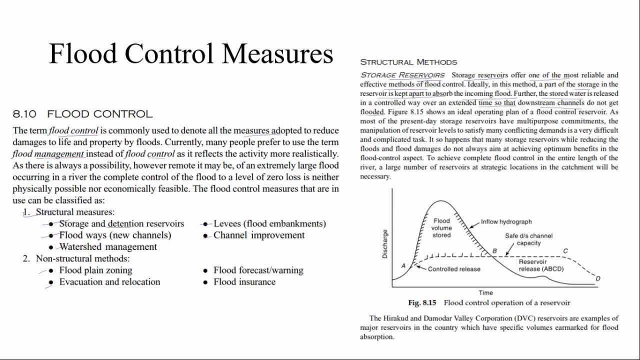 the downstream channels do not get flood. it is a simple example, so there can be other purposes. there can be multi purposes. you can make electricity canals etc. water can be used for flood damage. so it is like multi purpose things mostly. we adopt Hirakond in Damodar valley. 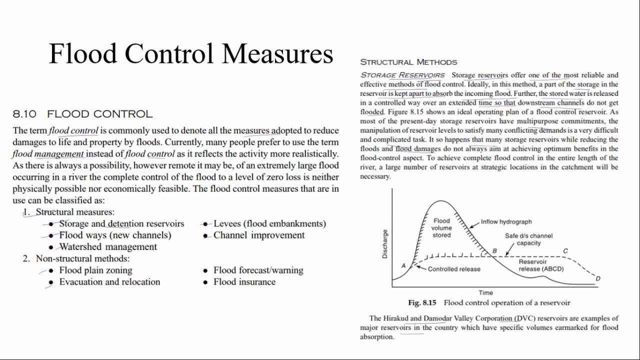 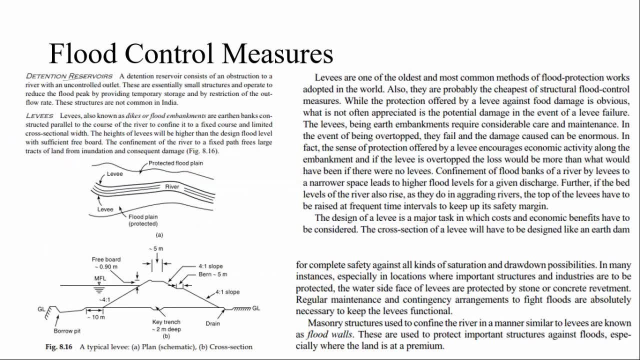 corporation is one of the major reservoir in the country, specifically for the flood absorption. now details: retention reservoir and flood storage reservoir. there is not much difference. retention means for small time period only. it blocks, it obstructs the river with an uncontrolled outlet in our country. there is not much. 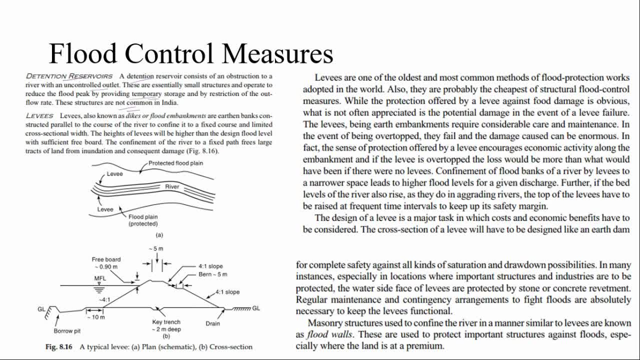 but in some countries it is used for temporary purpose. then there are levees, dikes or flood embankments, they are called. around the river. you make levee, you raise it, just like an other dam. you make a levee. so this is the flow of the river. 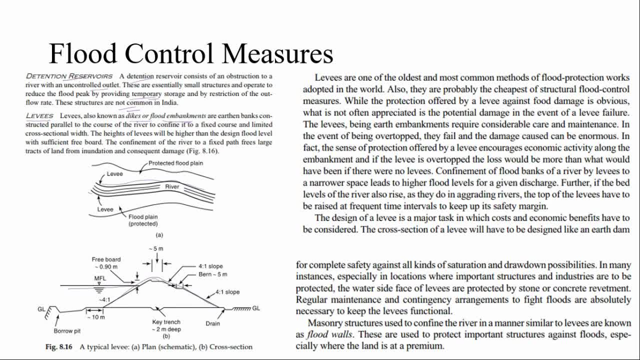 so, according to the high flood level, we have made this earthen dam. so along the river it flows. so what will happen? water will not go out of the flood plain. this confines the river to a fixed path. so they are one of the oldest method, most common method of. 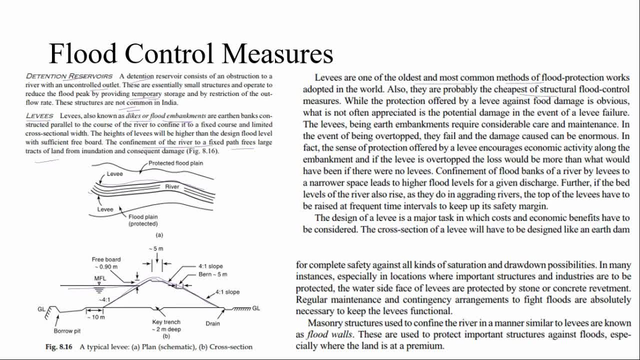 flood protection works, probably the cheapest of structural flood control measures. while the protection offered by levee is obvious, there can be some potential damage if levee fails because earthen dams can fail. if there is a failure from the side, then there can be flooding situation in case the sense of protection offered by levee 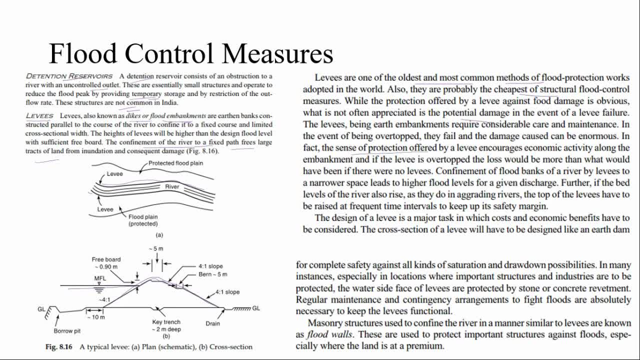 increases economic activity along the embankment. if the levee is over topped, the loss would be more than that would have been. but no levee. if the water flows at once, then there is no other loss. but the loss will increase. so the design of a levee is a major task. 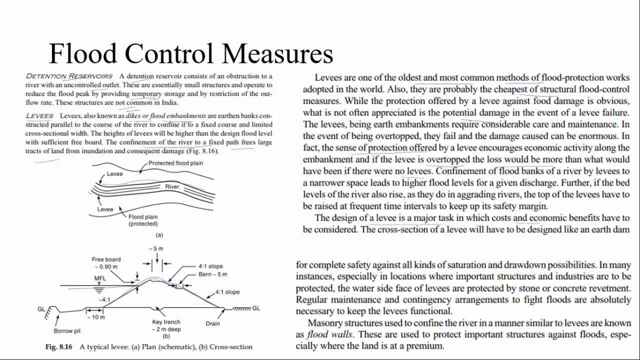 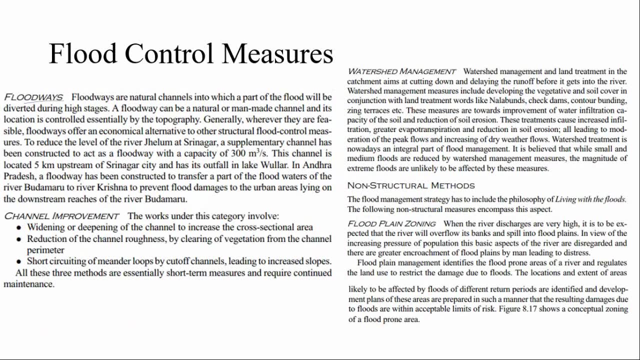 in which cost and economy have to be considered. so many times we use imaginary structures like flood walls. so instead of other dams, you can use imaginary structures. then there are some flood ways. flood ways are: we make natural channels in a part of the flood where there is a chance of flood. 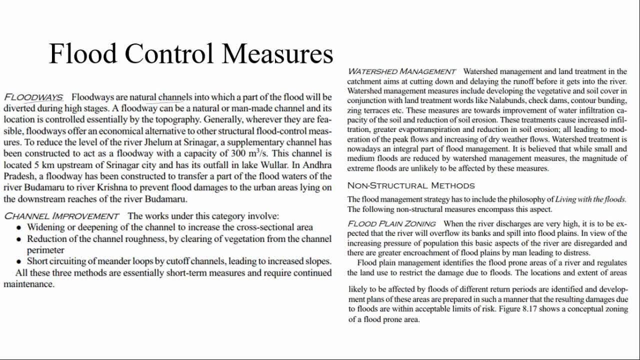 we make some natural pathways so when there is a flooding situation we can flow through those. for example, in chhelan river in srinagar, a supplementary channel has been constructed to act as a flood way. its capacity is 300 q max, located 5 km upstream of srinagar city. 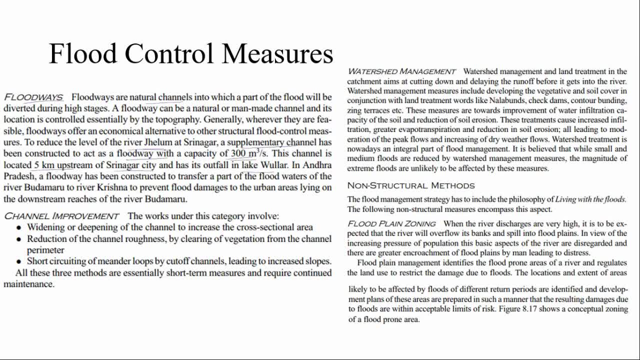 has its outfall in lake gular, so its water falls in lake gular. in case there is a flooding situation in andhra pradesh, there is an example. there are other measures also, what we can do. we can do widening or deepening of the channel. 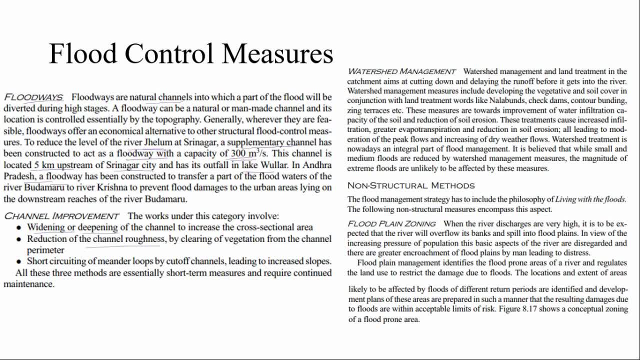 so that it can handle the flood. we can reduce the roughness of the channel so that there is vegetation in the channel so that more water can be accumulated. short circuit of meander loops by cut off channels in case of meander. sometimes the river passes through the city. 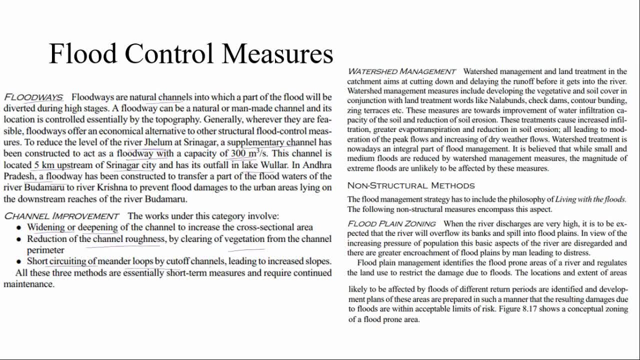 so by short circuit you can reduce its effect so that it stays away from the city. so there are also short term measures and what we can do is watershed management. what we do in this we are just cutting down and delaying the runoff before it gets into the river. 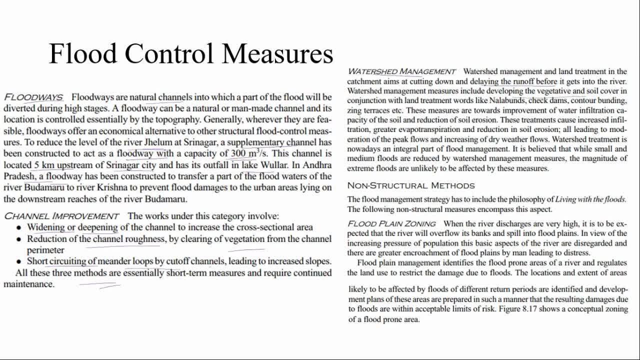 basically we have to delay the river. so what we do? we put a vegetable soil cover in the land treatment, so the area of the watershed from where the water is coming. you put a vegetable cover, trees, ponds, check dams, all these things- you can stop the peak flow of water. 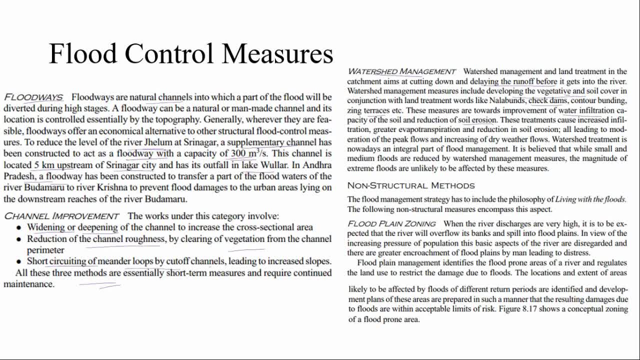 increase the water capacity, reduce the erosion of the soil, increase the precipitation, increase the evaporation, reduce the soil erosion. so all these things reduce the peak flow, especially in the dry weather. these are very important. then we have some non structural methods. so what we do in this? 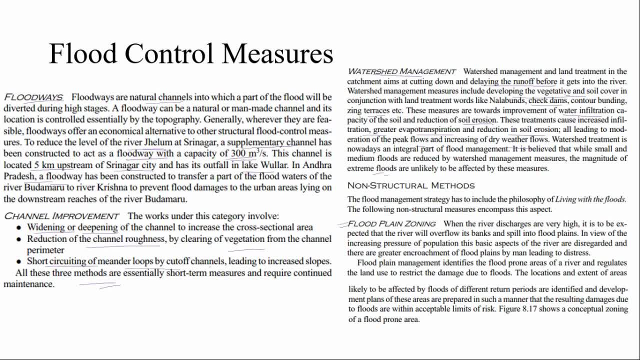 flood plain zooning. we map different different areas in flood plain zooning where the earth is zooned. it is zooned in different different cities. when the river discharge is very high, it is expected the river will overflow its banks and spill into 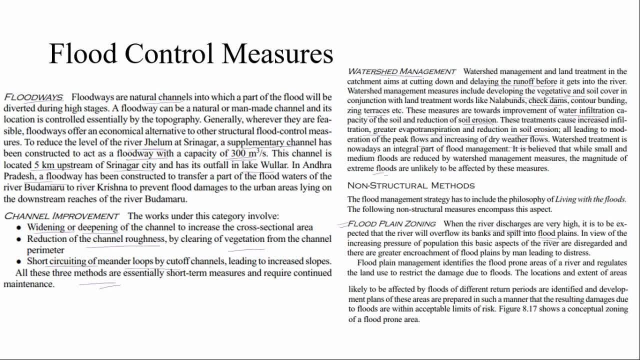 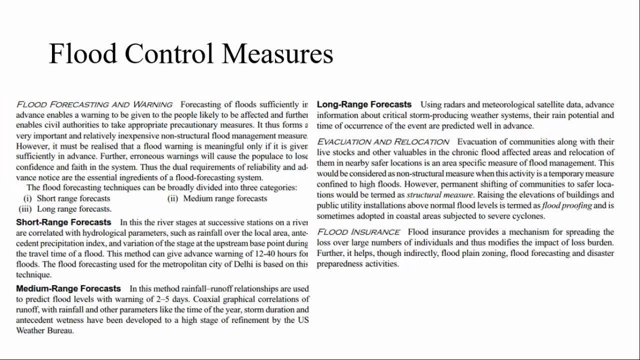 flood plains. so by doing such modelling, we can define the flood zone. then we have flood forecasting. so do the forecasting of the flood as simple as that. in advance, you forecast a warning signal for the people likely to be affected, so that enables civil authorities to take appropriate